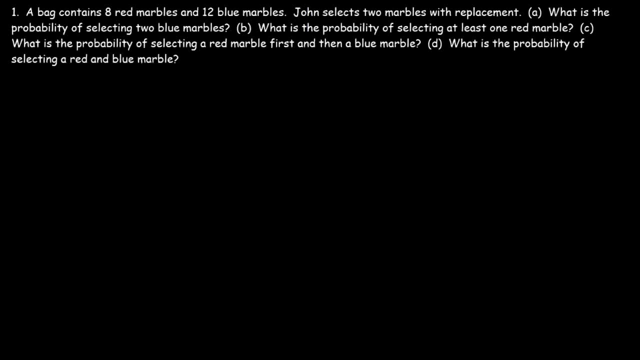 In this video we're going to talk about how to use tree diagrams to solve probability problems like this one. So we have a bag that contains eight red marbles and twelve blue marbles, and two marbles are selected with replacement. So part A: what is the probability of selecting two blue marbles. So let's. 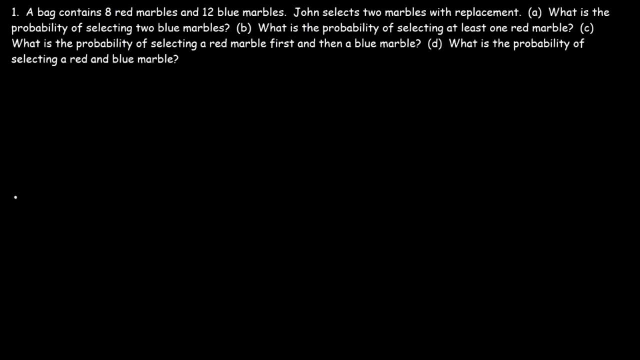 begin by drawing the tree diagram. So during the first selection there's two options. Either a red marble is selected or a blue marble. Now, if we select a red marble in the first try, in the second try it can be red or it can be blue. Now, 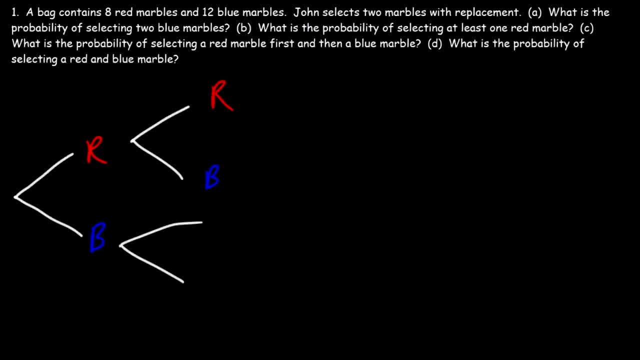 if we select a blue marble on the first try, on the second try it could be red or it could be blue. So thus we're going to get four possible outcomes If we go in this direction. the first outcome is red, and then red. If we 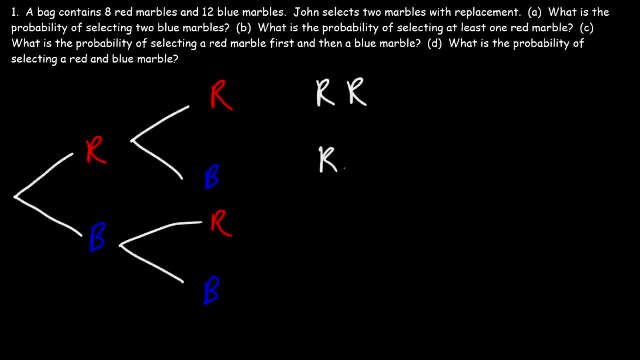 go in this direction. the second outcome is red and then blue. Or, if we go in that direction, it could be blue first and then red, Or, if we go in this direction, it can be blue and then blue. Now let's write down the numbers. So what is the probability of selecting a? 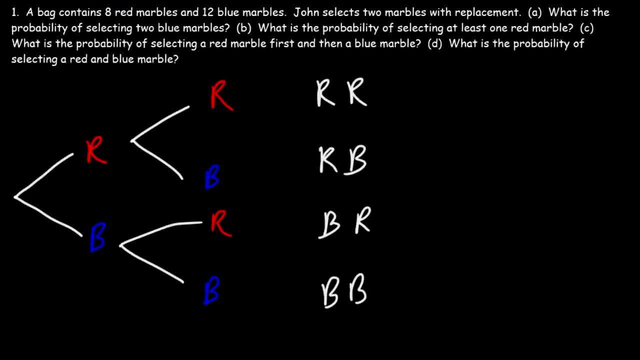 red marble. There's a total of 20 marbles. 8 are red, 12 are blue. So the probability of selecting a red marble on the first try is 8 out of 20.. And we can reduce this if we divide by 4.. So this becomes 2 over 5.. So that is the. 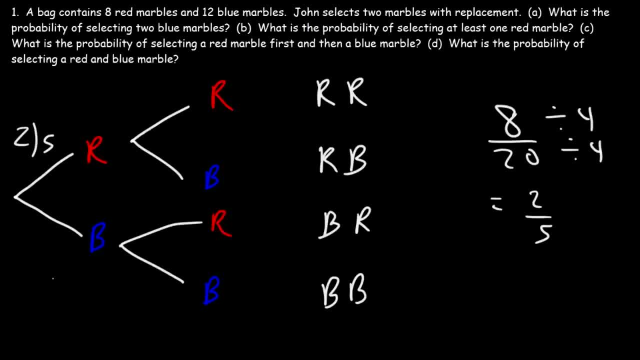 probability of selecting a red marble. Now the probability of selecting a blue marble. there's 12 blue marbles out of 20. And if we reduce the fraction this will be 3 over 5.. Now the problem says with replacement. So what that means is once you select a red marble or blue marble, 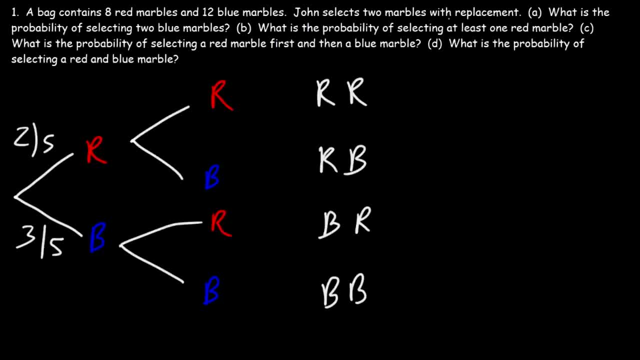 Now the problem says whiff replacement. So what that means is, once you select a red marble or blue marble on the first try, when you make your second selection you're going to put back the first marble in the bag. So that's the probability of selecting a red marble on the first try. 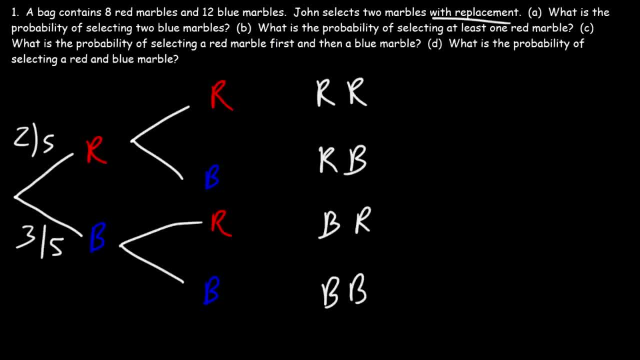 So you're still going to have a total of 20 marbles. So the probability of selecting another red marble is still 8 out of 20 or 2 out of 5.. And the probability of selecting a blue marble is still 12 out of 20 or 3 out of 5.. 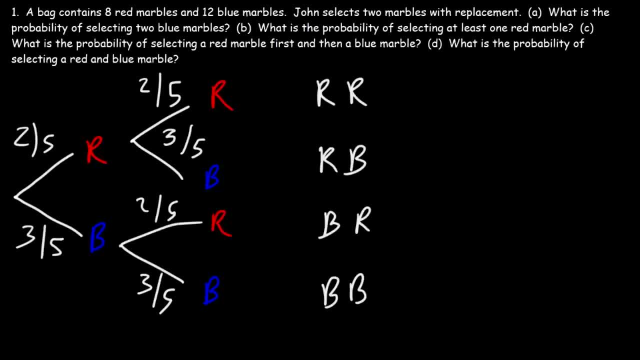 Now let's calculate the probability that corresponds to each outcome. So what is the probability of getting a red on the first try and another red on the second try? Now just to review whenever you hear the word and when you're connecting to events, 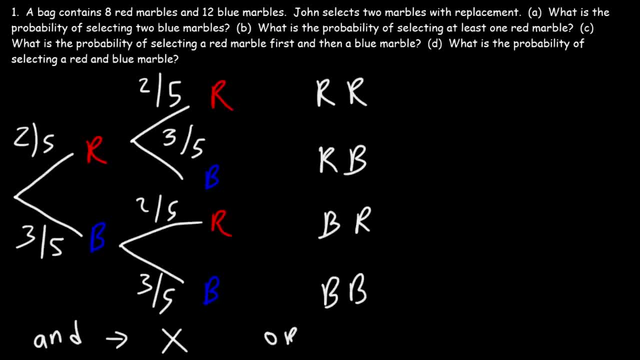 you need to multiply When you hear the word or you need to add. So we need to multiply these two numbers: 2 over 5 times 2 over 5.. 2 over 5 times 2 over 5. That's going to give us 4 over 25.. 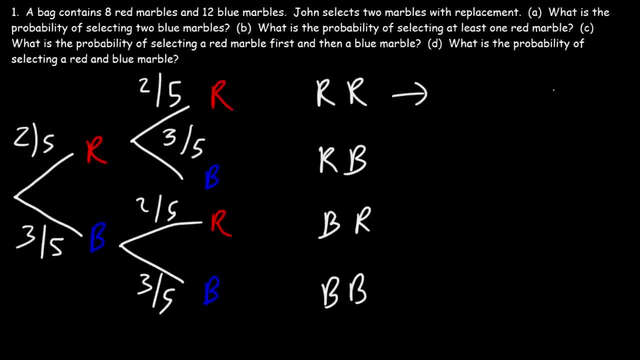 So the probability of selecting a red marble and then another red marble is going to be 4 over 25.. What about red and then blue? So we need to go in this direction. Thus, we need to multiply 2 over 5 by 3 over 5.. 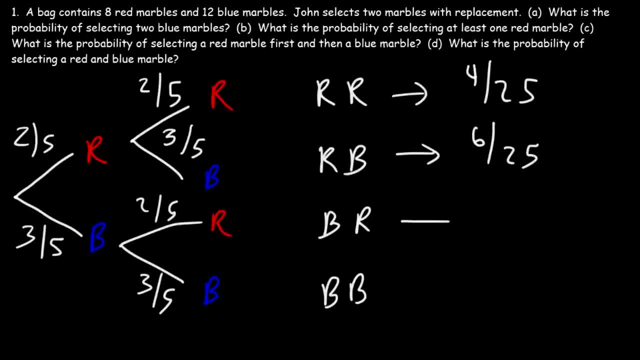 And that's going to give us 6 over 25.. And for blue and then red it's also going to be the same thing, That's 6 over 25.. And then the probability of selecting 2 blue marbles is going to be 3 over 5 times 3 over 5.. 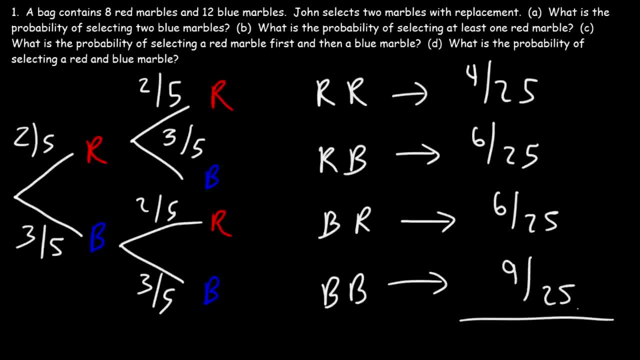 Which is 9 over 25.. Now, if we add up these four values, it should give us 1.. 4 plus 6 is 10.. Plus 6, that's 16. Plus 9, that's 25.. 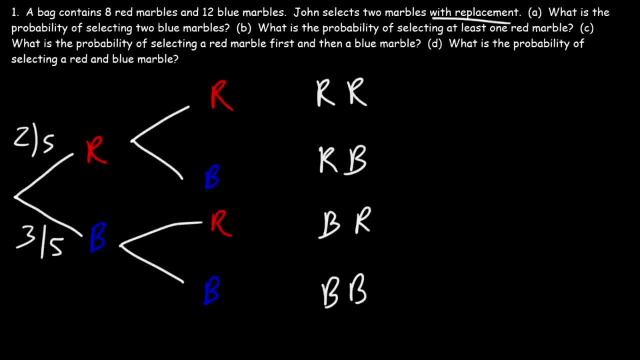 on the first try. when you make your second selection, you're going to put back the first marble in the bag, So you're still going to have a total of 20 marbles. So the probability of selecting another red marble is still 8 out of 20, or 2 out of 5.. And the 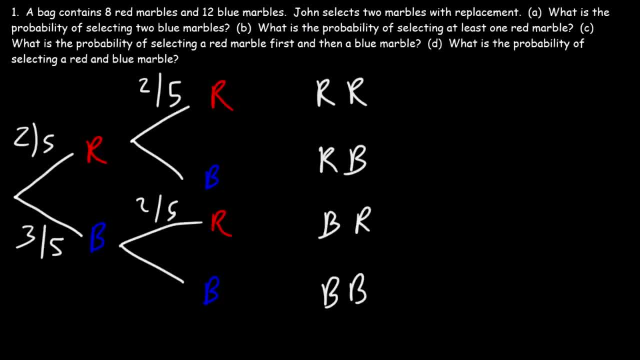 probability of selecting a blue marble is still 12 out of 20, or 3 out of 5.. Now let's calculate the probability that corresponds to each outcome. So what is the probability of getting a red on the first try AND another red on? 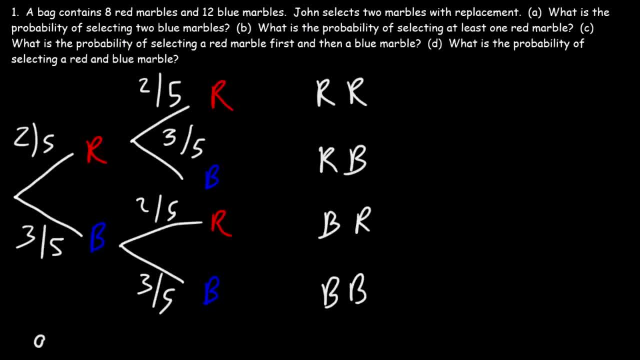 a second try Now just to review. whenever you hear the word and when you're connecting two events, you need to multiply When you hear the word or you need to add. So we need to multiply these two numbers Two over five times. 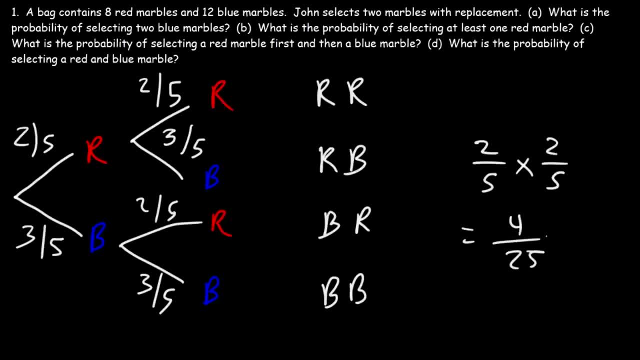 2 over five. that's going to give us 4 over 25.. So the probability of selecting a red marble and then another red marble is going to be 4 over 25.. What about red and then blue? So we need to go in this direction. 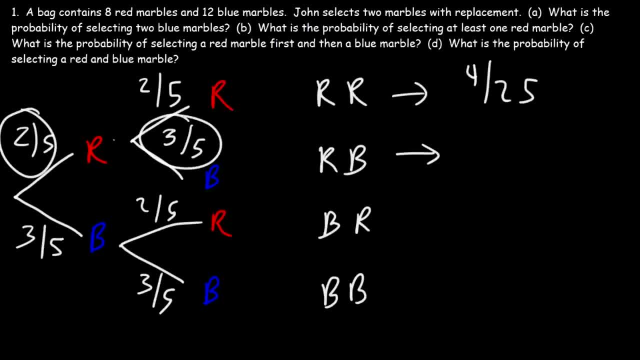 thus we need to multiply 2 over 5 by 3 over 5, and that's going to give us 6 over 25.. And for blue and then red it's also going to be the same thing, that's 6 over. 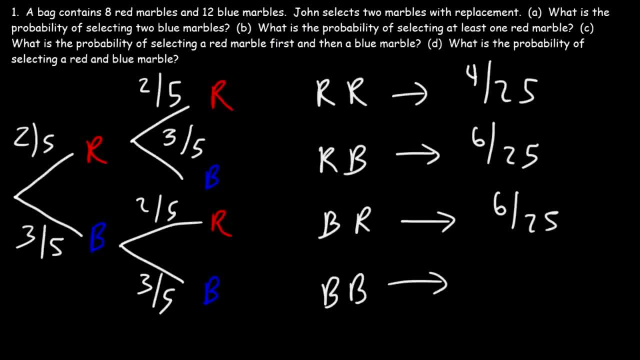 25.. And then the probability of selecting 2 blue marbles is going to be 3 over 5 times 3 over 5, which is 9 over 25.. Now if we add up these four values, it should give us 1.. 4 plus 6 is 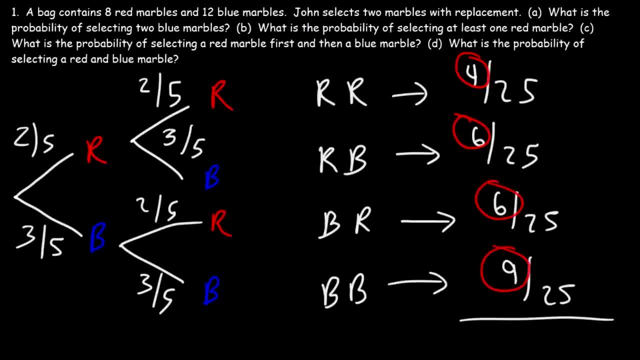 6.. 10 plus 6,, that's 16, plus 9,, that's 25.. So we get 25 over 25, which is 1.. And 1 corresponds to 100%. So now that we've completed the tree diagram, we can now. 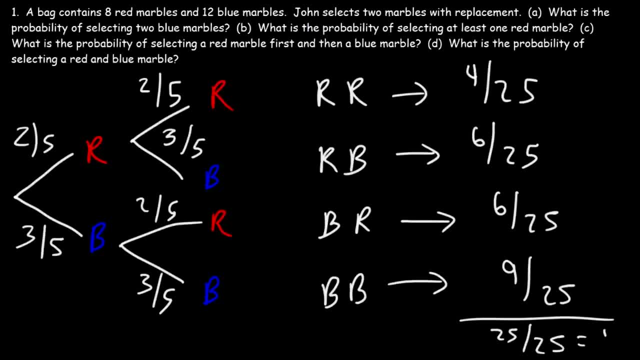 So we get 25.. Over 25,, which is 1., And 1 corresponds to 100 percent. So now that we've completed the tree diagram, we can now answer the questions in this problem. So what is the probability of selecting 2 blue marbles? 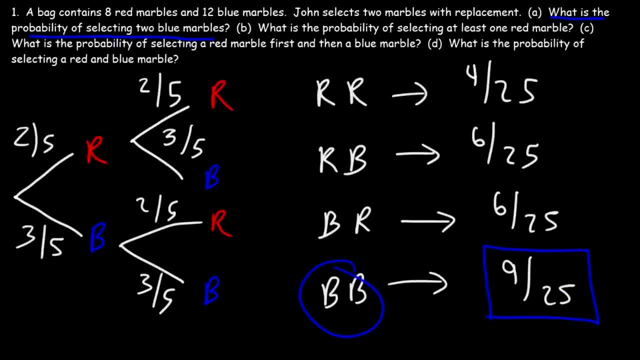 So the answer is right here. The probability of selecting 2 blue marbles is 9 over 25.. Now if you want to turn that into a decimal value, you can type that into a calculator. 9 divided by 25 as a decimal is 0.36.. 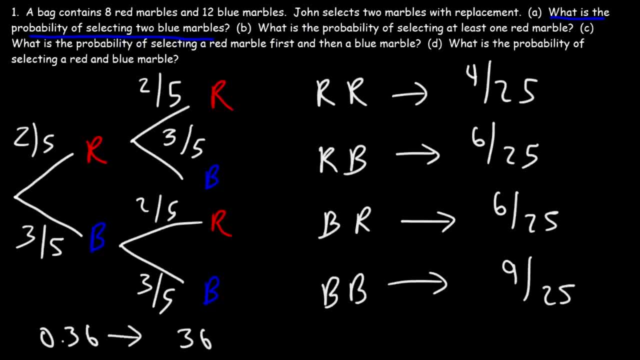 And if you multiply that by 100, you get 36 percent. So there's a 36 percent chance of selecting 2 blue marbles. So that's the answer for part A. Now part B: What is the probability of selecting at least 1 red marble? 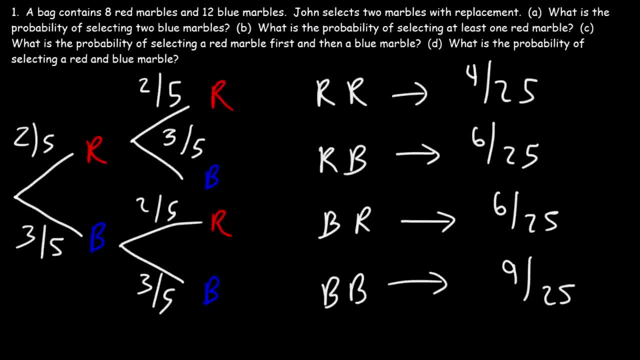 So think about that. How can we find the answer? Looking at the four possible outcomes, which ones contain at least 1 red marble? So this one has at least 1 red marble, And the same is true for that one and this one. 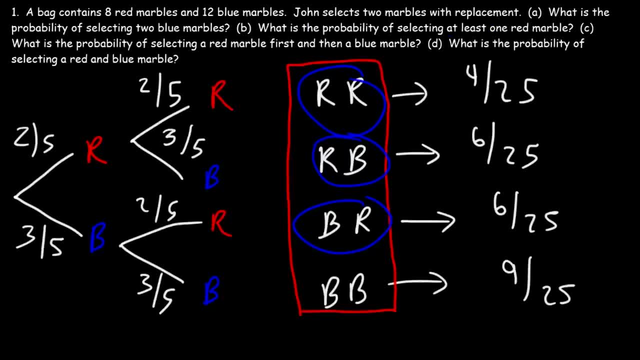 So, in order to calculate the probability of selecting at least 1 red marble, what we need to do is add up these three values, Because it could be RR or RB or BR, And remember the word OR when dealing with probability means that you need to add the. 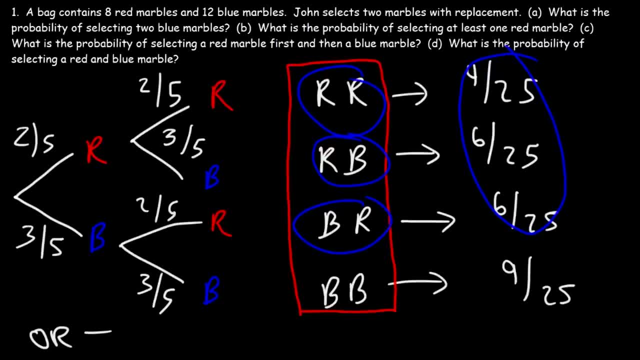 individual probabilities for each event. So it's going to be 4 over 25, plus 6 over 25, plus another 6 over 25.. And so that's going to be 16 over 25, which is 0.64 or 64 percent. 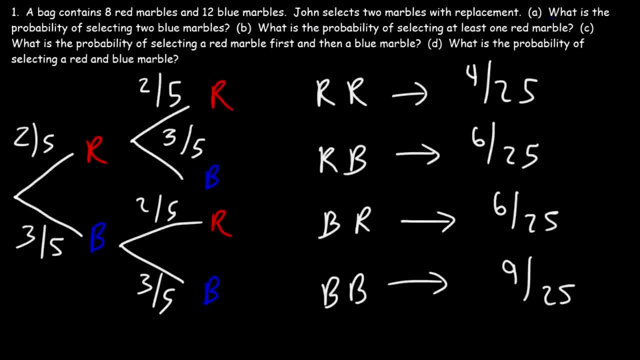 answer the questions in this problem. So what is the probability of selecting 2 blue marbles? So the answer is right here: The probability of selecting 2 blue marbles is 9 over 25.. Now if you want to turn that into a decimal value, you can type that into a. 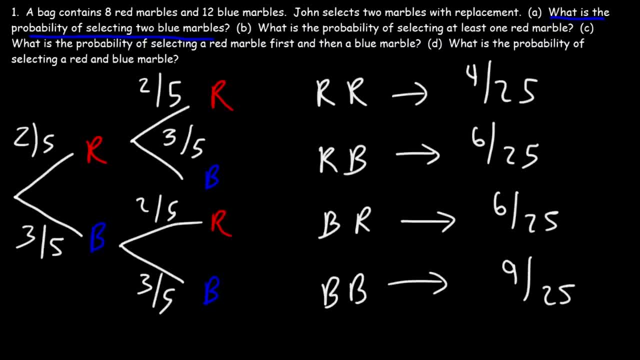 calculator: 9 divided by 25 as a decimal is 0.36.. And if you multiply that by 100, you get 36%. So there's a 36% chance of selecting 2 blue marbles. So that's the answer for part A. Now part B: What is the probability of? 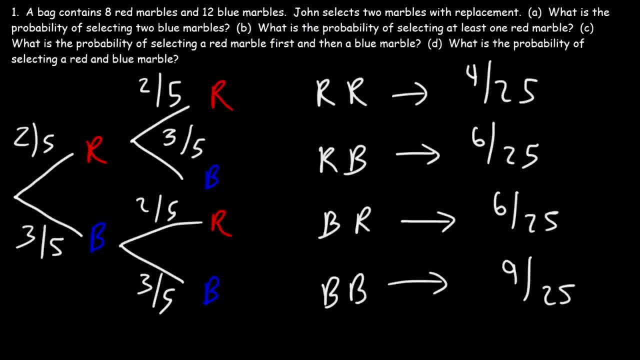 selecting at least 1 red marble. So think about that. How can we find the answer? Looking at the four possible outcomes, which ones contain at least 1 red marble? So this one has at least 1 red marble, And the same is true for that. 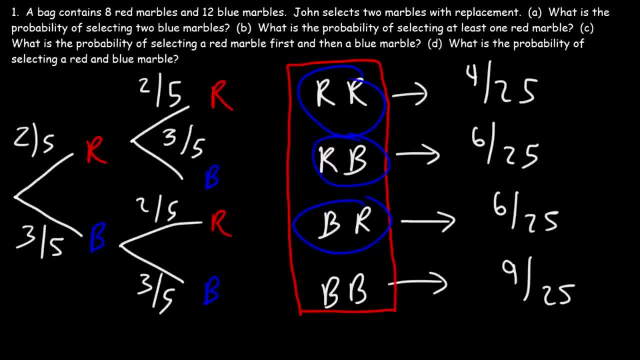 one and this one. So, in order to calculate the probability of selecting at least 1 red marble, what we need to do is add up these three values, Because it could be RR or RB or BR, And remember the word OR. 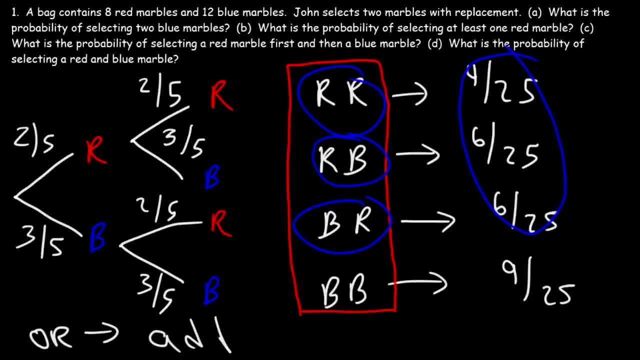 when dealing with probability means that you need to add the individual probabilities for each event. so it's going to be 4 over 25 plus 6 over 25, plus another 6 over 25, and so that's going to be 16 over 25. 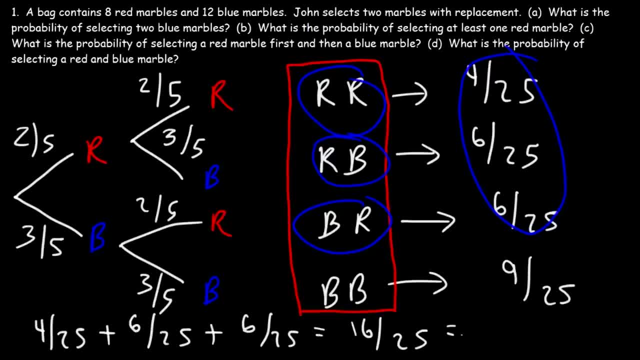 which is 0.64 or 64 percent. now there's another way in which you can get the same answer, and it's important to understand that the probability of selecting at least one red marble is equal to the probability of not selecting two blue marbles. 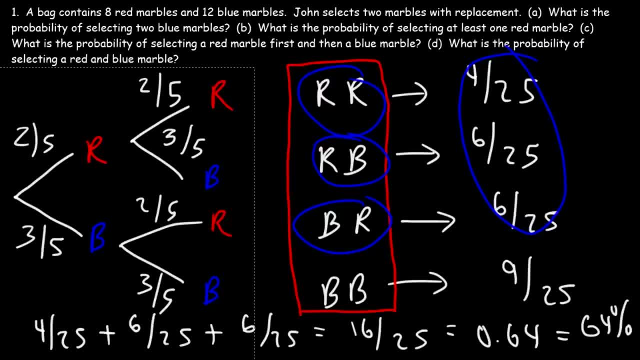 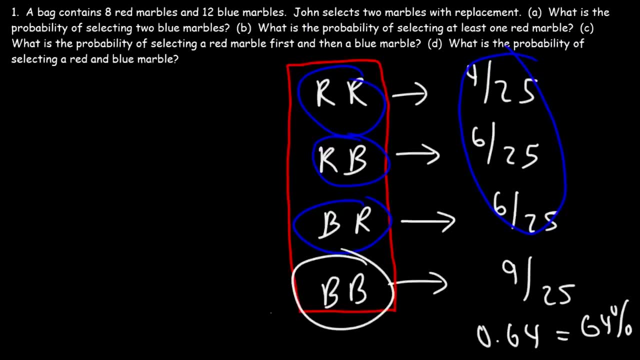 Now there's another way in which you can calculate the probability of selecting at least 1 red marble. This one is RR And it's the same answer, And It's important to understand that the probability of selecting at least 1 red marble is equal to the probability of not selecting 2 blue marbles. 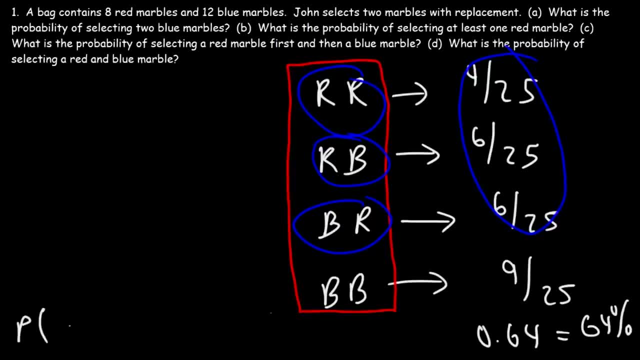 So understanding that you can use this formula. So the probability of getting at least 1 red marble- let's say R is 0.64, 2 red marbles is 0.64, 0.64.. So that's the probability of getting at least 1 red marble. 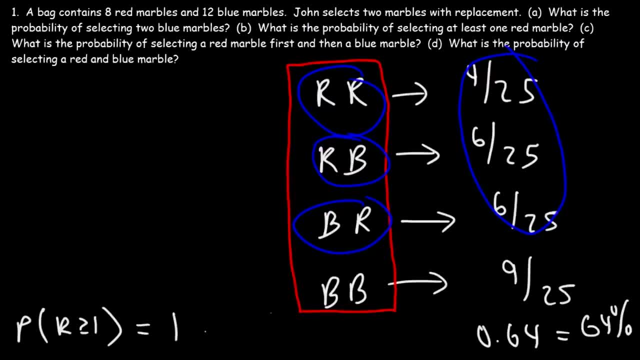 is equal to a greater than 1. it's equal to the probability of not getting two blue marbles, which is 1 minus the probability of getting two blue marbles. so the probability of an event occurring is equal to 1 minus the probability of that event not occurring. so this is going to be 1 minus 0.36, which is the. 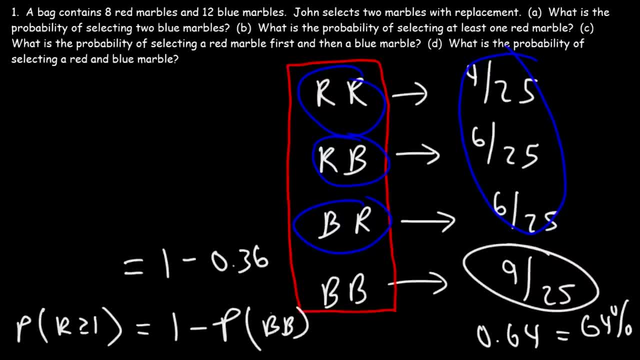 answer that we had in part 8, the probability of getting two blue marbles was 9 over 25, which is 0.36, and 1 minus 0.36 is 0.64, which gives us 64% again. so that's the other way in which you can get the same answer. now let's move. 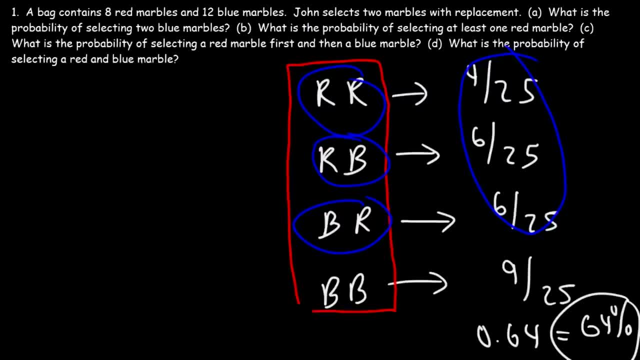 on to the next part, part C. what is the probability of selecting a red marble first and then a blue marble? so the answer is just 6 over 25 and as a decimal that's 0.24, which corresponds to 24%. So that's it for Part C. Now Part D: what is the probability of selecting a red marble? 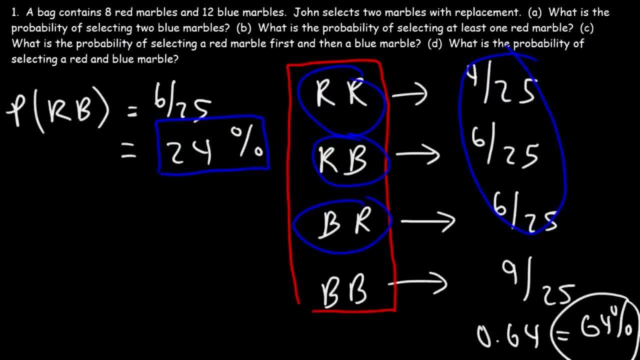 and a blue marble. Think about that. So I'm going to give you a minute to think about how to do it. Feel free to pause the video and tell me what you think. the answer is for Part D, or at least write it down and play the video to see if you have it right. 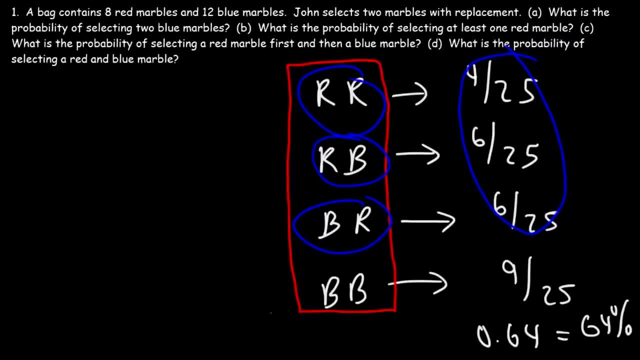 so understanding that you can use this formula. so the probability of getting at least one red marble, let's say r, is equal to a greater than one. it's equal to the probability of not getting two blue marbles, which is one minus the probability of getting two blue marbles. 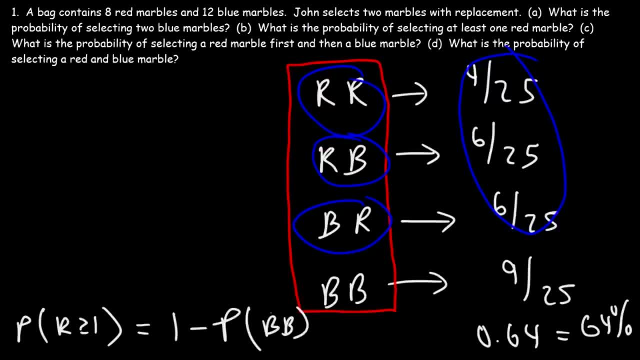 so the probability of an event occurring is equal to one minus the probability of that event not occurring. so this is going to be 1 minus 0.36, which is the answer that we had in part eight. the probability of getting two blue marbles was 9 over 25, which is 0.36, and 1 minus 0.36 is 0.64. 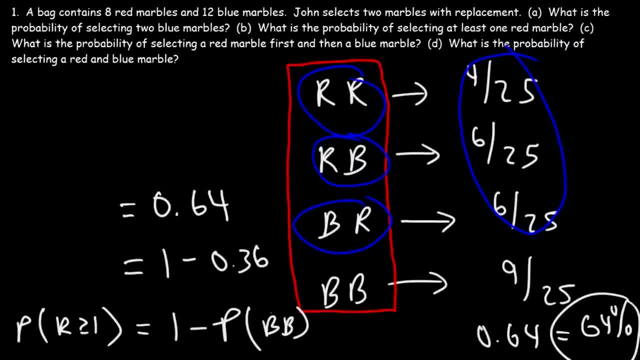 which gives us 64 percent again. so that's the other way in which you can get the same answer. now let's move on to the next part, part c. what is the probability of selecting a red marble first and then a blue marble? so the answer is just: 6 over 25. 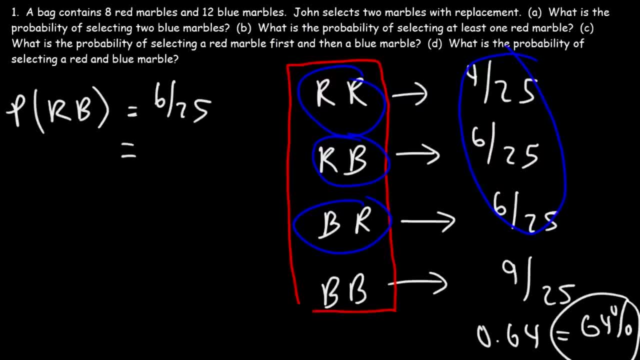 and as a decimal, that's the probability of selecting a red marble first and then a blue marble: 0.24, which corresponds to 24%. So that's it for part C. Now part D: what is the probability of selecting a red marble and a blue marble? Think about that, So I'm going to give you a minute. 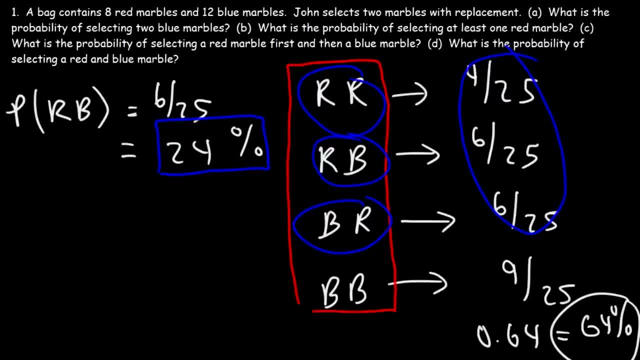 to think about how to do it. Feel free to pause the video and tell me what you think the answer is for part D, or at least write it down and play the video to see if you have it right. In part C, the order of selecting the two marbles matter In part D. 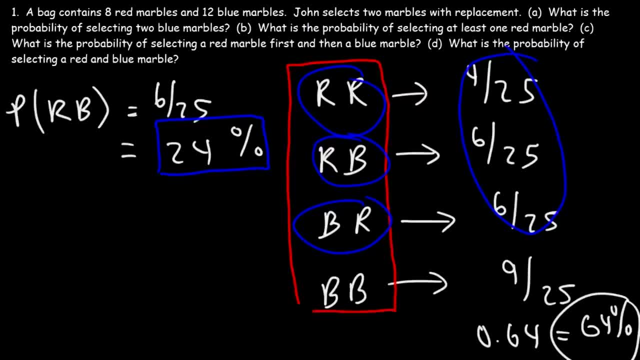 the order does not matter, And that's the key difference between part C and D. So for part C it has to be red first and then blue, So that's only RB. But in part D we just need a red and blue marble, So that could be RB. 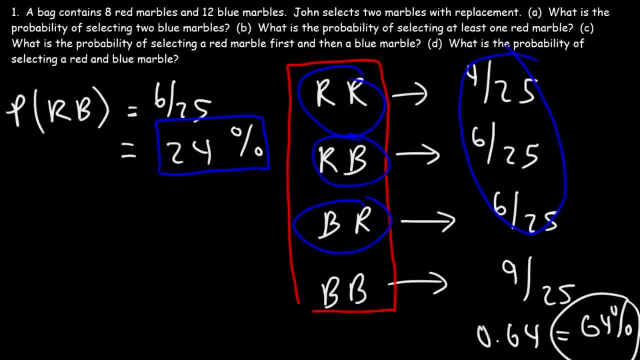 In Part C the order of selecting the two marbles matter. In Part D the order does not matter, And that's the key difference between Part C and D. So for Part C it has to be red first and then blue, so that's only RB. 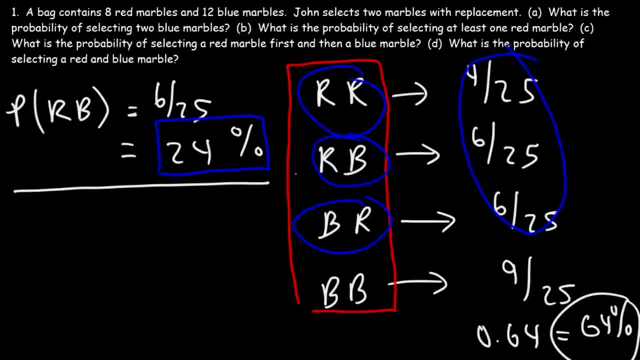 But in Part D we just need a red and blue marble, So that could be RB or BR, Because they both contain a red and a blue marble. So we need to add these two values, 6 over 25, plus another 6 over 25, that's 12 over 25,, which is .48, or 48%. 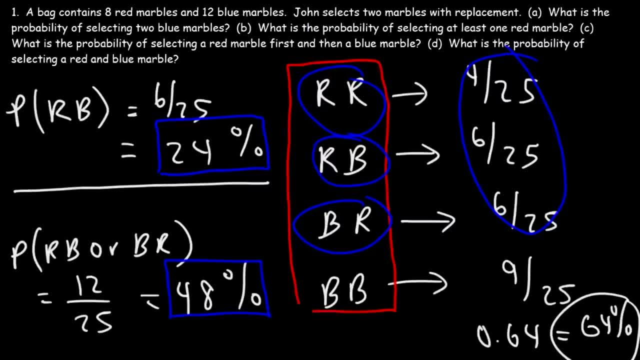 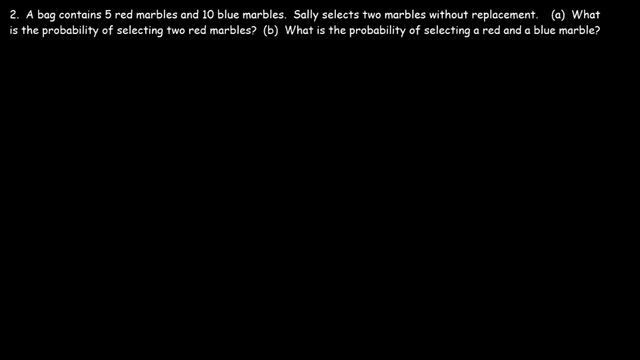 So there's a 48% chance of selecting a red and a blue marble, but there's a 24% chance of selecting a red marble first And then a blue marble. So be careful with questions like that. Now let's work on this question. 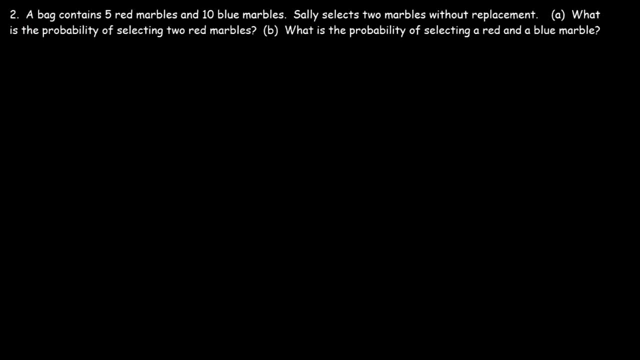 A bag contains 5 red marbles and 10 blue marbles. Sally selects 2 marbles without replacement. What is the probability of selecting 2 red marbles? So let's begin by making our tree diagram. So the first two options that we can get is either going to be a red marble or a blue. 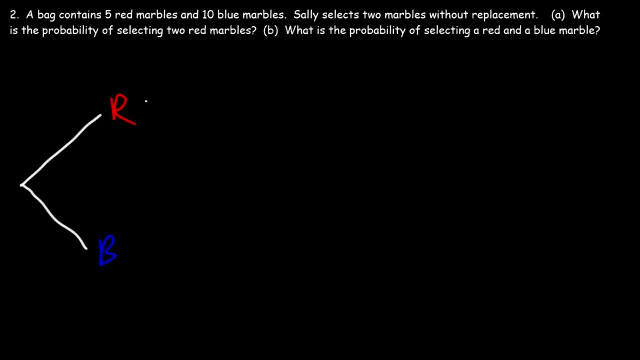 marble on the first try. Now, if we get a red marble on the first try, then we can either get another red or a blue, just like before. And if we get a blue on the first try, we can get a red on the second try or another. 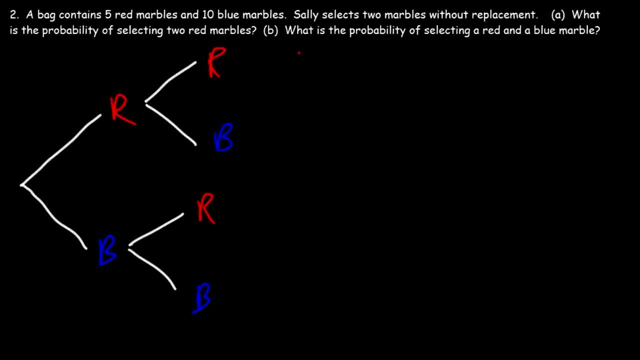 blue marble. So the first options could be. So the first options could be R R and the second option could be R B. The third outcome will be B R and the fourth outcome B B. Now what is the probability of selecting a red marble? So we have five. 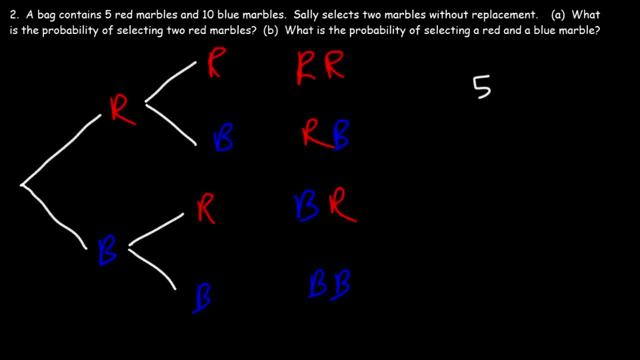 red marbles and ten blue marbles. So it's going to be five red marbles out of a total of 15, and if we divide both numbers by five we can reduce it to one over three. Now the probability of selecting a blue marble on the first try: there's ten blue marbles out. 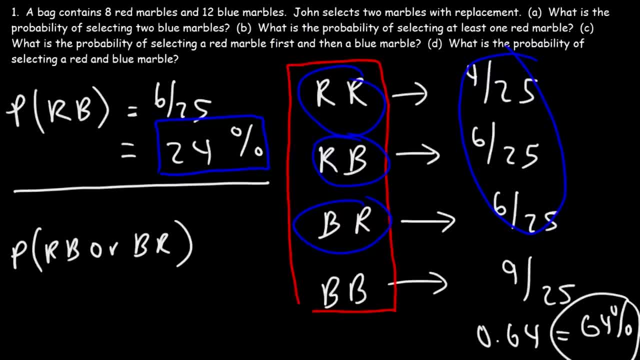 or BR, because they both contain a red and a blue marble. So we need to add these two values, 6 over 25, plus another 6 over 25, that's 12 over 25, which is 0.48, or 48%. 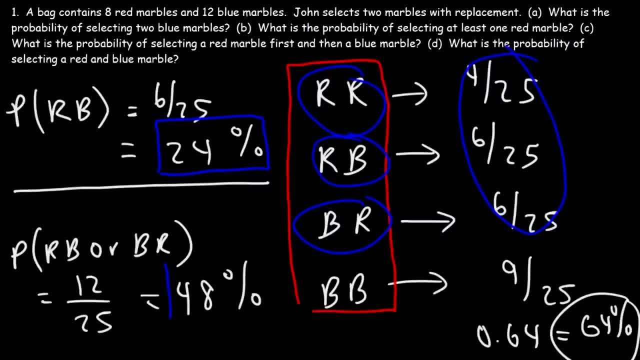 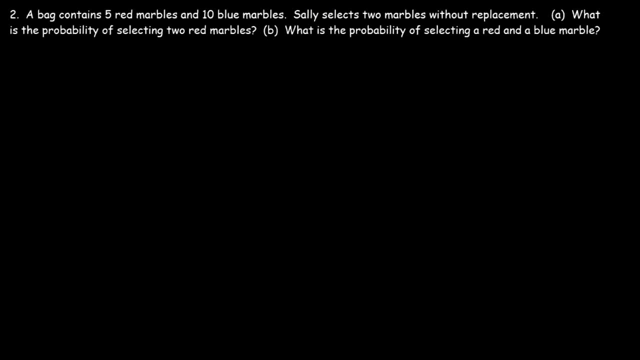 So there's a 48% chance of selecting a red and a blue marble, but there's a 24% chance of selecting a red marble first and then a blue marble. So be careful with questions like that. Now let's work on this question. 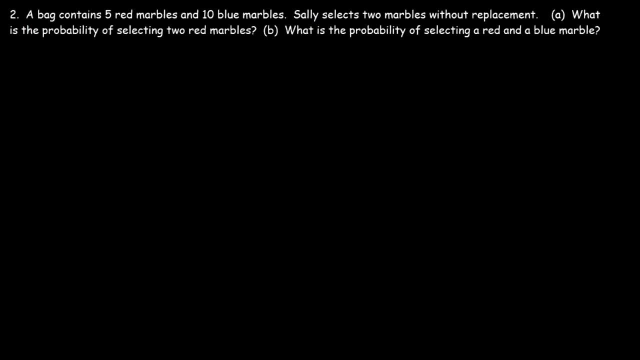 A bag contains 5 red marbles and 10 blue marbles. Sally selects 2 marbles without replacement. What is the probability of selecting 2 red marbles? So let's begin by making a guess. We're making our tree diagram. 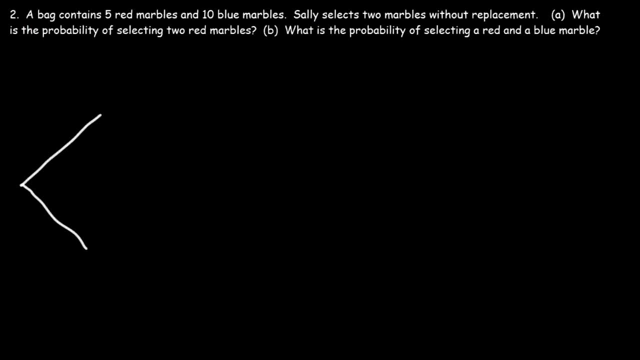 So the first two options that we can get is either going to be a red marble or a blue marble on the first try. Now, if we get a red marble on the first try, then we can get either another red or a blue, just like before. 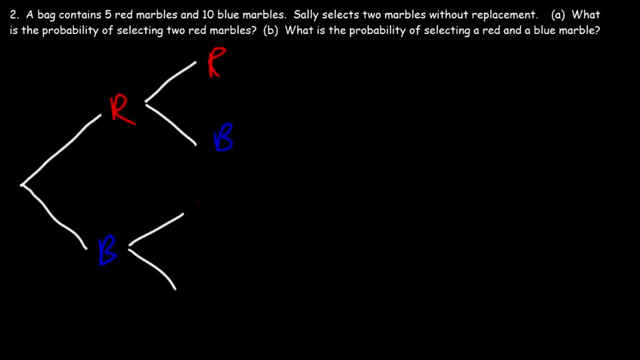 And if we get a blue on the first try, we can get a red on the second try or another blue marble. So the first option could be RR and the second option could be RB, The third outcome will be BR and the fourth outcome BB. 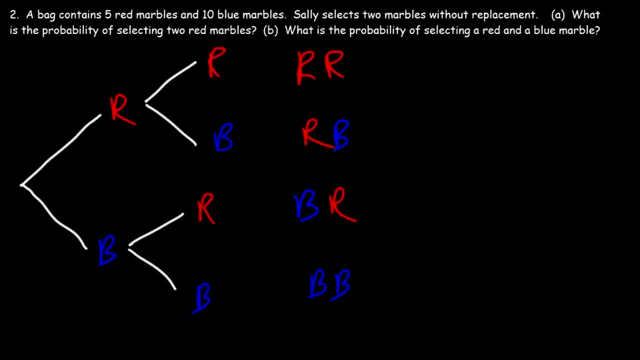 Now what is the probability of selecting a red marble? So we have 5 red marbles and 10 blue marbles, So it's going to be 5 red marbles out of a total of 15, and if we divide both numbers by 5, we can reduce it to 1 over 3.. 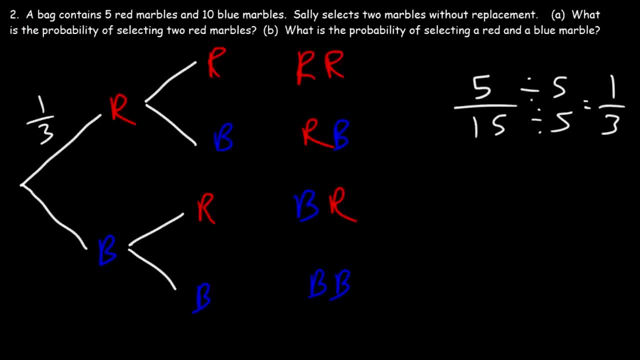 Now the probability of selecting a blue marble on the first try. there's 10 blue marbles out of 15, and so we can reduce this fraction to 2 over 3.. Now what about the probability of selecting a red marble on the second try? 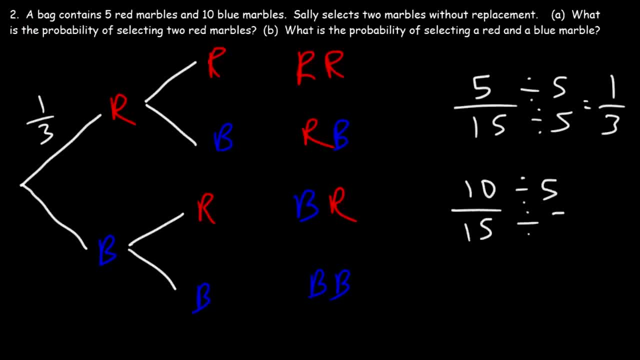 of 15, and so we can reduce this fraction to two over three. Now, what about the probability of selecting a red marble on the second? try Now remember: this problem is without replacement. So what does that mean? It means that when Sally selects the first marble, she doesn't put it back in the bag before selecting the. 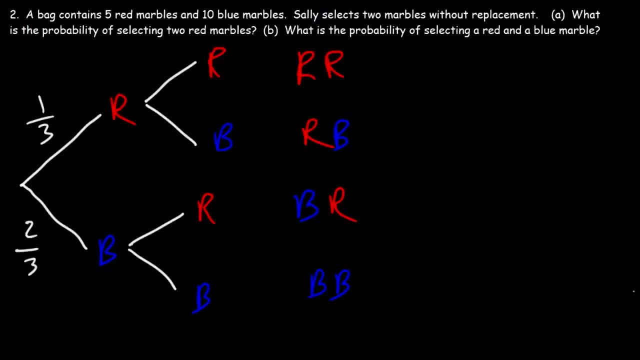 second marble. So during the second try we're not going to have a total of 15 marbles, we're going to have a total of 14 marbles, because she took out one. she took out a red marble. so now we have four red marbles and 10 blue marbles. so this is what. 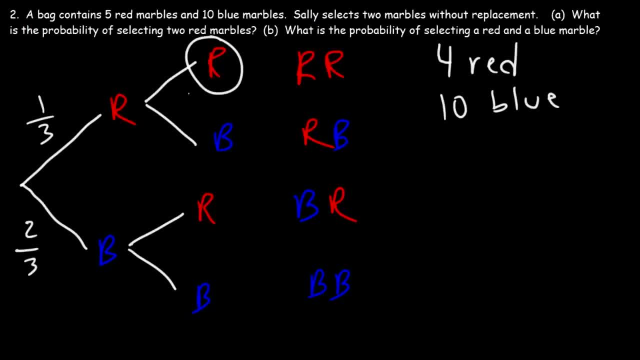 is known as dependent events, because the second event depends on the first event, whether she took out a red or blue. in the last problem, there were independent events. the second event did not depend on the first event. now, if she takes out a blue marble, what just happened there? 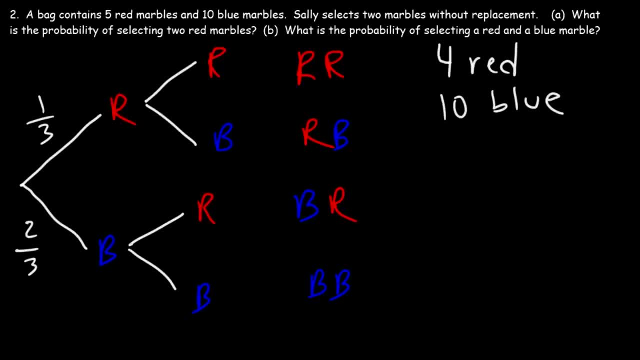 if Sally takes out a blue marble on the first try, there's going to be five red marbles left over and nine blue marbles left over for the second try. so, as you can see this, the amount of marbles, or rather the type of marbles that will have, is dependent on the first event. so 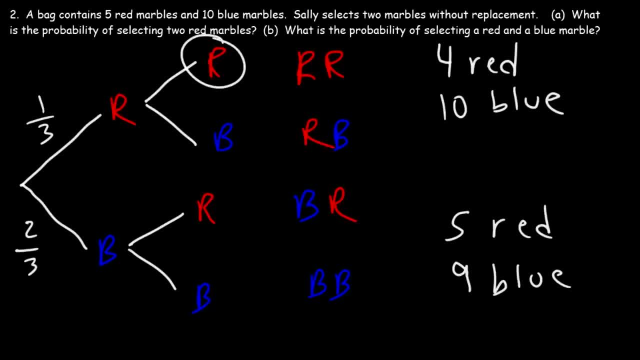 over here. what is the probability of selecting a red marble during the second event? so we have four red marbles out of a total of 14. so it's four out of 14, and if we divide both numbers by two we can reduce that to two over seven. so on the second try, the probability is: 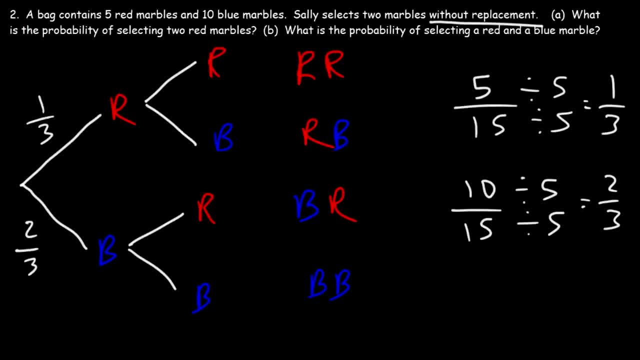 Now remember: this problem is without replacement. So what does that mean? It means that when Sally selects the first marble, she doesn't put it back in the bag before selecting the second marble. So during the second try we're not going to have a total of 15 marbles out of 15.. 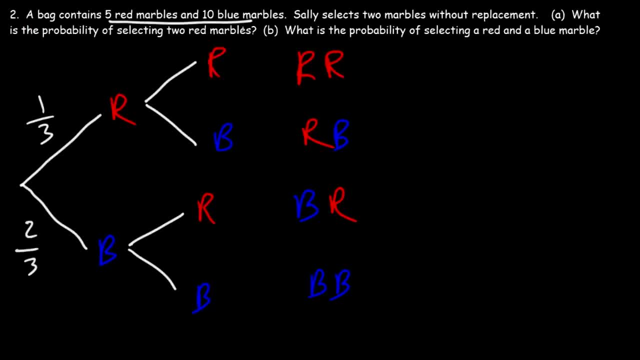 We're going to have a total of 14 marbles. because she took out one. So in the first try she took out a red marble. So now we have 4 red marbles and 10 blue marbles. So this is what is known as dependent events, because the second event depends on the first event, whether she took out a red or a blue. 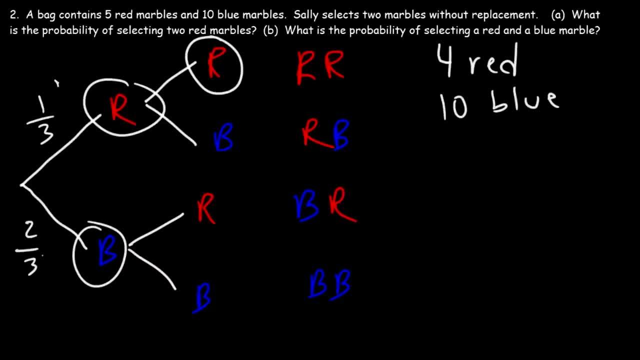 In the last problem there were independent events. The second event did not depend on the first. Now, if she takes out a blue marble- what just happened there- If Sally takes out a blue marble on the first try, there's going to be 5 red marbles left over and 9 blue marbles left over for the second try. 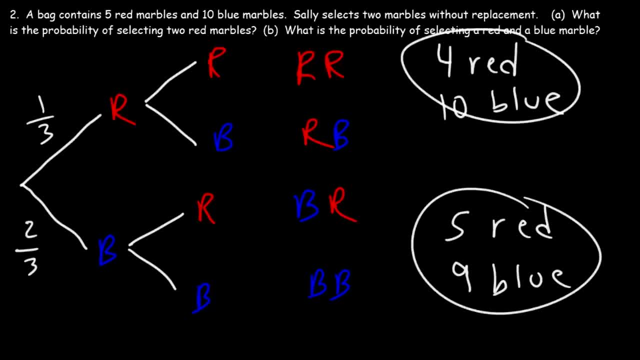 So, as you can see, the amount of marbles, or rather the type of marbles that we'll have, is dependent on the first event. So, over here, what is the probability of selecting a red marble during the second event? So we have 4 red marbles out of a total of 14.. 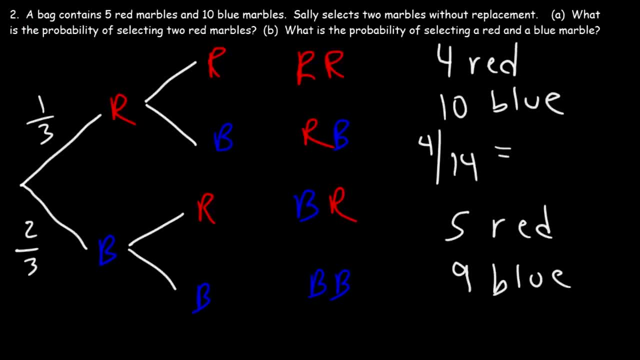 So it's 4 out of 14.. And if we divide both numbers by 2, we can reduce that to 2 over 7.. So on the second try, the probability is 2 over 7 that a red marble will be selected. 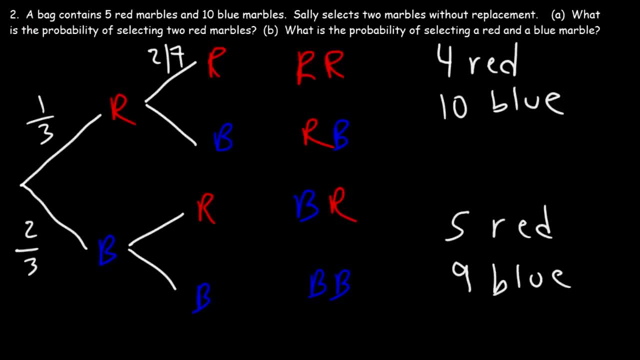 What about a blue marble? on the second? try Particularly this blue marble. So we have 10 blue marbles out of 14.. If we divide 10 and 14 by 2, that will be 5 over 7.. Notice that these two numbers add up to 1.. 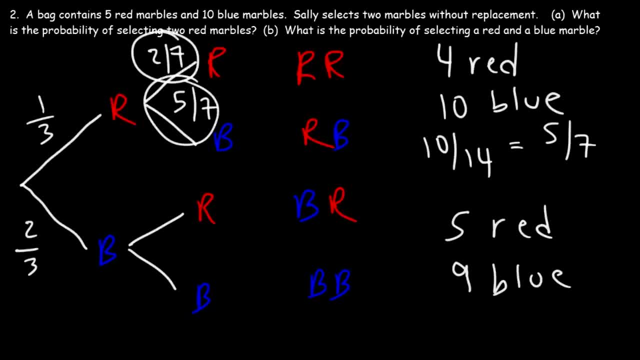 That's 3 over 3.. And these two numbers add up to 7 over 7,, which is 1.. The probability of an event happening or this event not happening, which is equal to the probability of that event happening, always adds up to 1.. 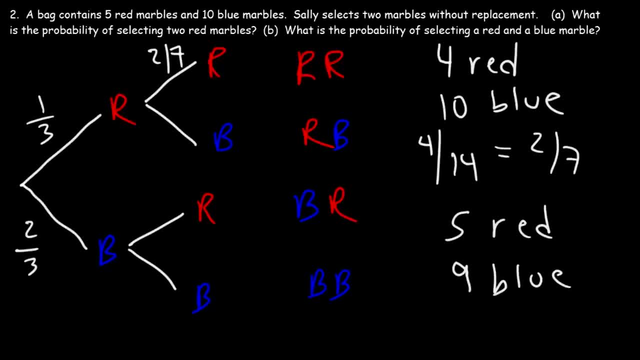 two over seven, that a red marble will be selected. what about a blue marble? on the second, try, particularly this blue marble. so we have 10 blue marbles out of 14. if we divide 10 and 18 by 2, that will be 5 over 7. notice that these two numbers add up to 1, that's 3 over 3. and these: 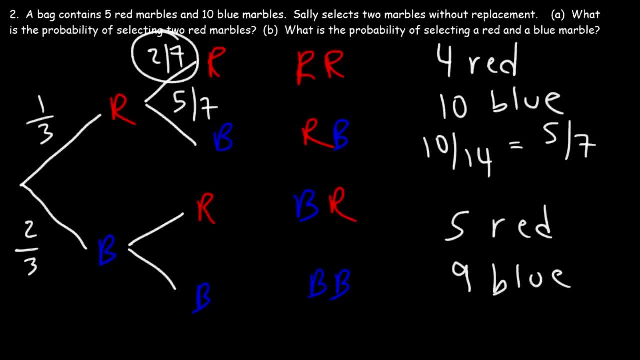 two numbers add up to 7 over 7, which is 1. the probability of an event happening or this event not happening, which is equal to the probability of that event happening, always adds up to 1. now let's look at the the other side. what is the probability of getting this particular red marble after we get? 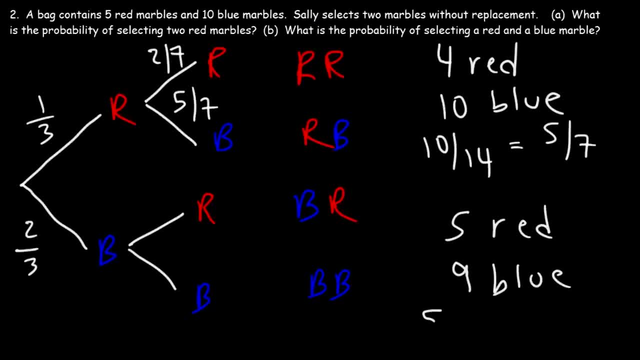 a blue marble on the first try. so now we have five red marbles out of a total 14. so it's just 5 out of 14. now the probability of selecting a blue marble on the second try after getting a blue marble on the first try. that's going to be nine blue marbles out of 14. 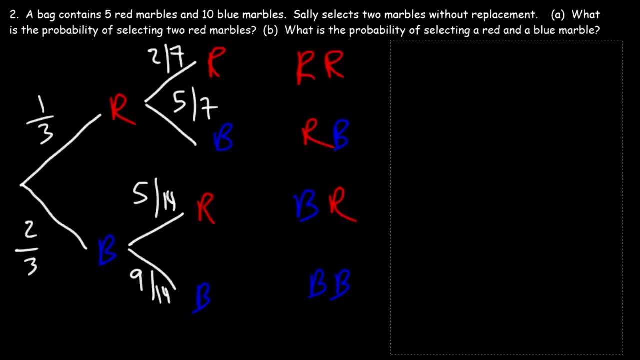 so now we can answer the questions part a: what is the probability of selecting two red marbles? so the probability of getting a red marble on the first try is 1 over 3, and then the probability of getting another red marble on the second try is 2 over 7. so we need to multiply those two numbers. 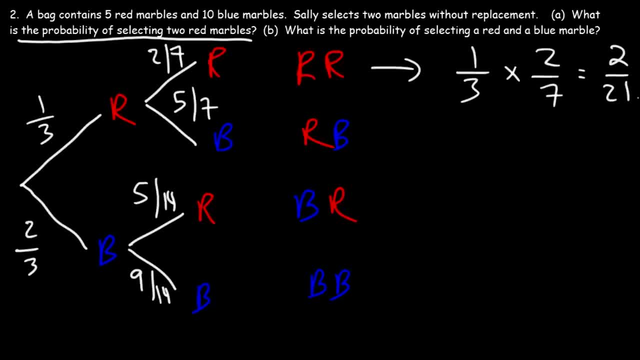 and this becomes 2 over 21, which is like 0.095238. so we could say it's approximately. there's a 9.5% chance of getting two red marbles. so that's the answer for part a or the approximate answer. part b: what is the? 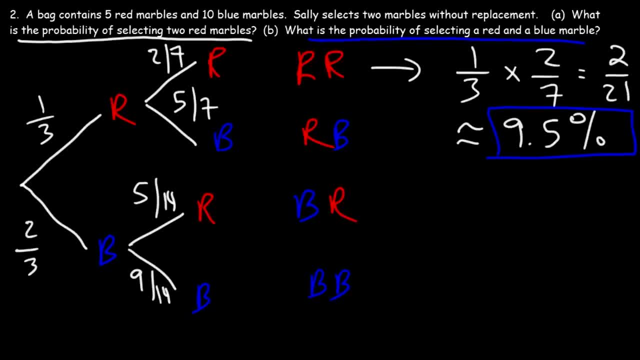 probability of selecting a red and a blue marble. so does the order matter here? are we looking for red and then blue, or are we looking for red, blue or blue and red? all we need is just a red and blue marble, so this is going to be the answer. so the probability of getting 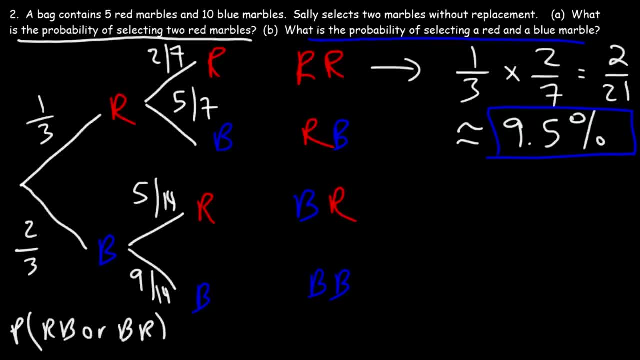 RB or BR is going to be the sum of the probabilities of those two events. so let's get PRB- the probability of getting R and then B plus the probability of getting B and then R. so let's start with this one. this is going to be 1 over 3 times 5 over 7. 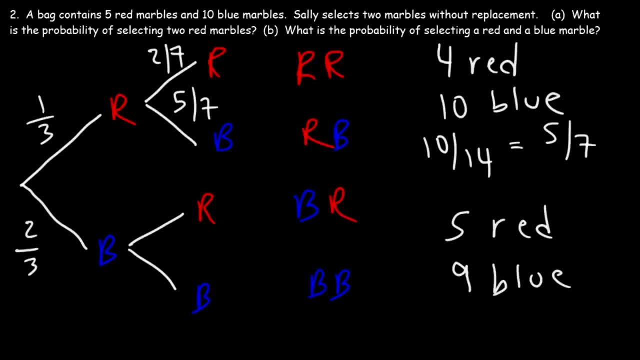 Now let's look at the other side. What is the probability of getting this particular red marble after we get a blue marble on the first try? So now we have 5 red marbles out of a total of 14.. So it's just 5 out of 14.. 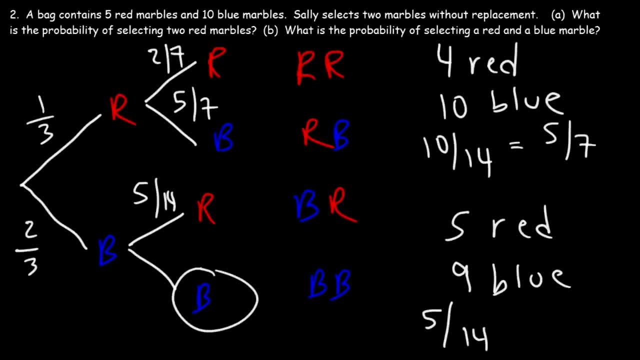 Now the probability of selecting a blue marble on the second try after getting a blue marble on the first try. that's going to be 9 blue marbles out of 14.. So now we can answer the questions Part A: What is the probability of selecting 2 red marbles? 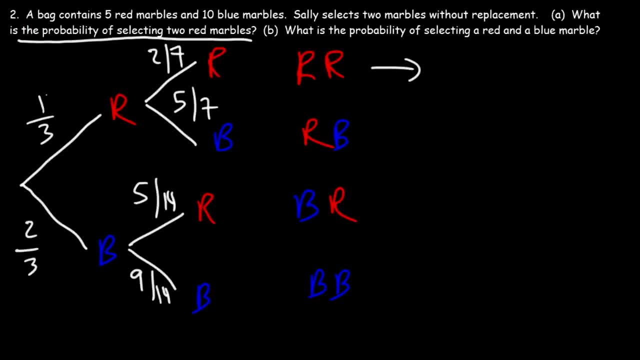 So the probability of getting a red marble on the first try is 1 over 3.. And then the probability of getting another red marble on the second try is 1 over 3.. And then the probability of getting another red marble on the second try is 2 over 7.. 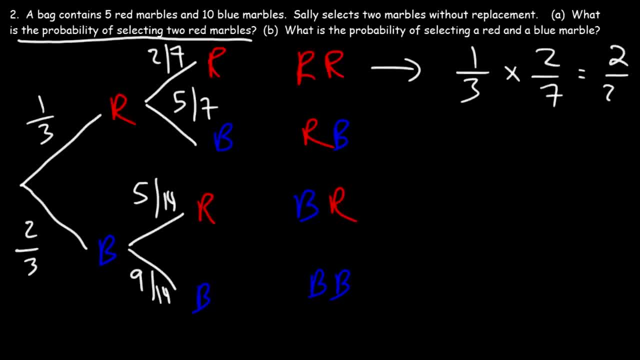 So we need to multiply those two numbers and this becomes 2 over 21.. Which is like .095238.. So we could say it's approximately: there's a 9.5% chance of getting 2 red marbles. So that's the answer for Part A, or the approximate answer. 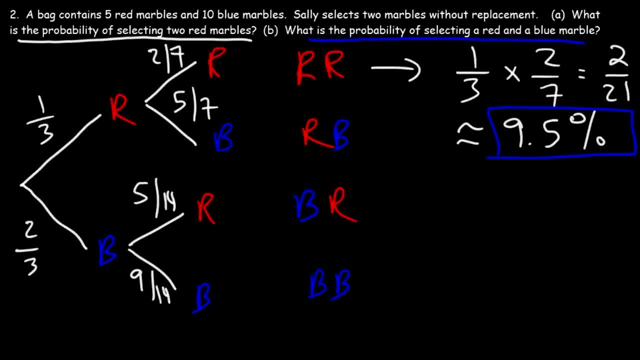 Part B: What is the probability of selecting a red and a blue marble? So does the order matter here? Are we looking for red and then blue, Or are we looking for red, blue or blue and red? All we need is just a red and blue marble. 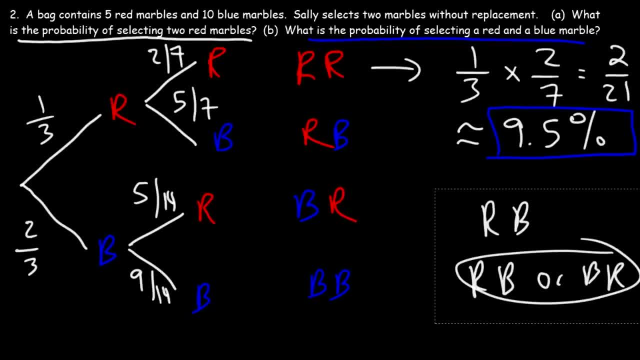 So this is going to be the answer: The probability of getting RB or BR is going to be the sum of the probabilities of those two events. So let's write PRB: the probability of getting R and then B, plus the probability of getting B and then R. 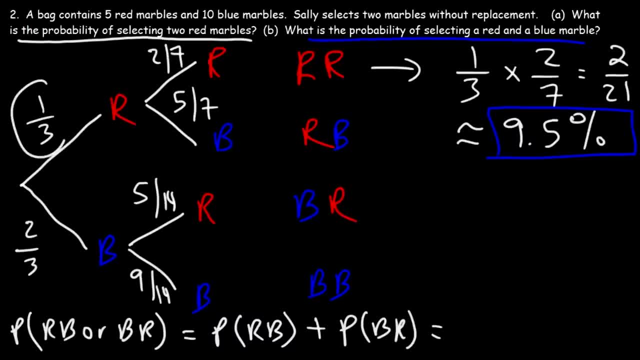 So let's start with this one. This is going to be 1 over 3 times 5 over 7.. And then for this one, it's going to be 2 over 3 times 5 over 14.. So this is the probability of getting RB. 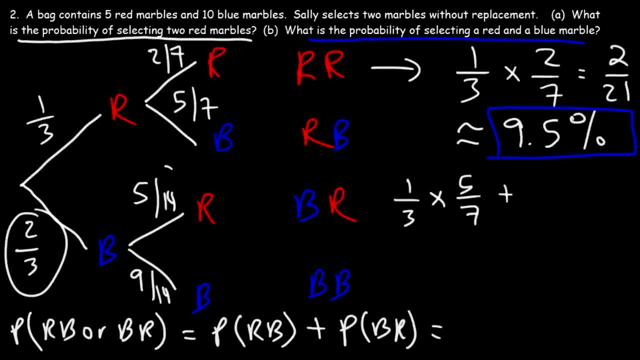 and then for this one, it's going to be 2 over 3 times 5 over 14, and then for this one, it's going to be 2 over 3 times 5 over 14. so this is the probability of getting RB and this represents the probability of. 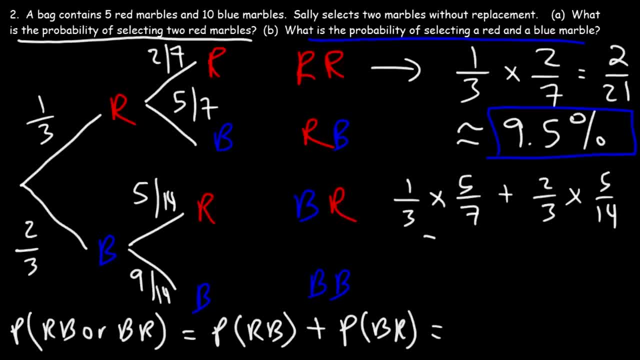 getting BR. so this is going to be 5 over 21. just multiply across and for the second part, 3 2 times 5 is 10. 3 times 4 is 42. but we can reduce that if you divide both numbers by 2. 10 divided by 2 is 5. 42 divided by 2 is 21. 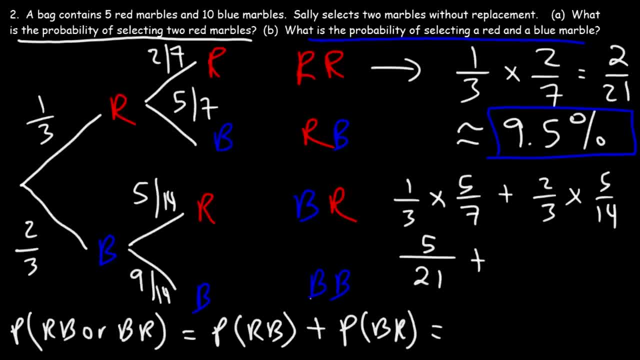 so that becomes 5 over 21. these two, it turns out they have the same probability, and so that gives us 10 out of 21, which is 0.47619. so this is going to be approximately 47.6 percent. so there's a 47.6 percent chance. 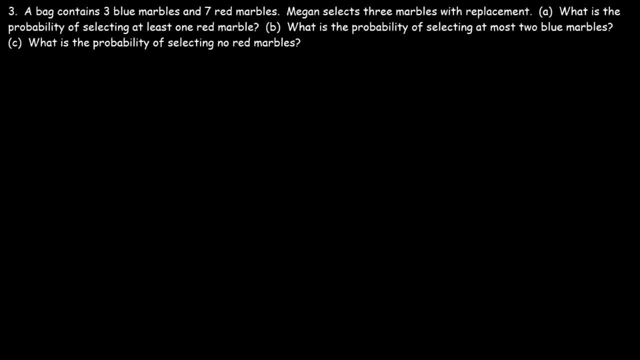 of getting a red and a blue marble. number three: a bag contains three blue marbles and seven red marbles. Megan selects three marbles with replacement. what is the probability of selecting at least one red marble? so let's begin with a tree diagram. as always, we have two options. on the first try, she can select. 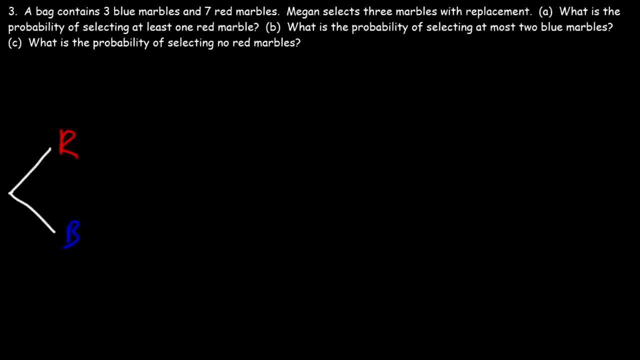 a tree diagram. as always, we have two options. on the first try, she can select a red marble or a blue marble, and on the second try- remember there's three selections- she's selecting three marbles. so on the second try, it can be red and blue again, and after selecting blue, it can also be red and blue again. now 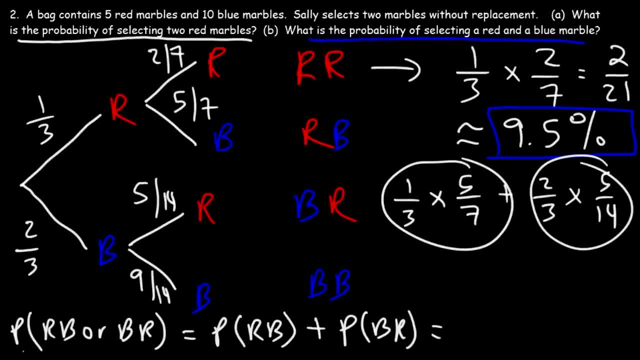 And this represents the probability of getting BR. So this is going to be 5 over 21.. Just multiply across And for the second part, 2 times 5 is 10.. 3 times 4 is 42. But we can reduce that. 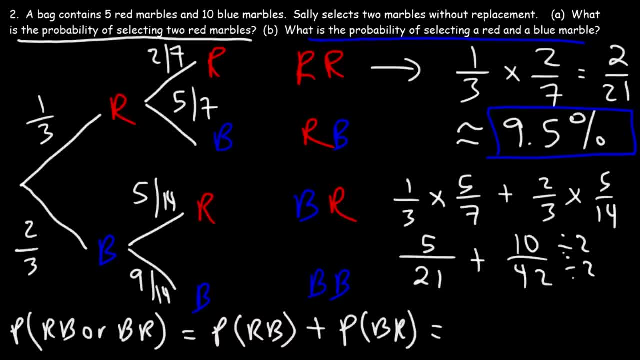 If you divide both numbers by 2,, 10 divided by 2 is 5.. 42 divided by 2 is 21.. So that becomes 5 over 21.. These two, it turns out they have the same probability, And so that gives us 10 out of 21.. 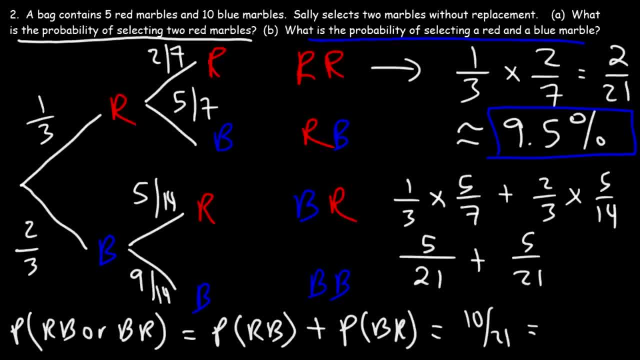 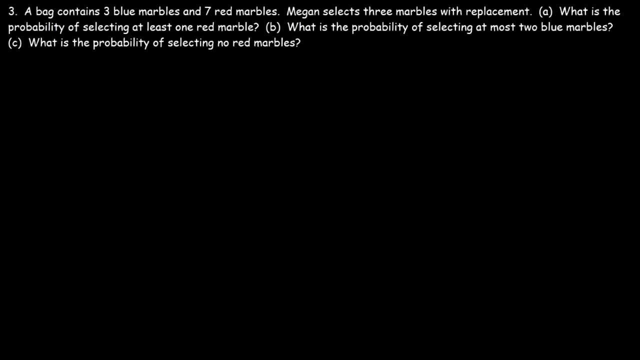 Which is 0.4.. So this is going to be approximately 47.6%. So there's a 47.6% chance of getting a red and a blue marble, Number 3.. A bag contains 3 blue marbles and 7 red marbles. 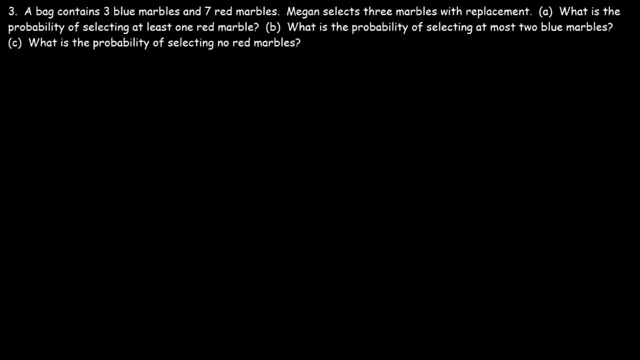 Megan selects 3 marbles with replacement, What's the probability of selecting at least one red marble? So let's begin with a tree diagram. As always, we have two options. On the first try, she can select a red marble or a blue marble. 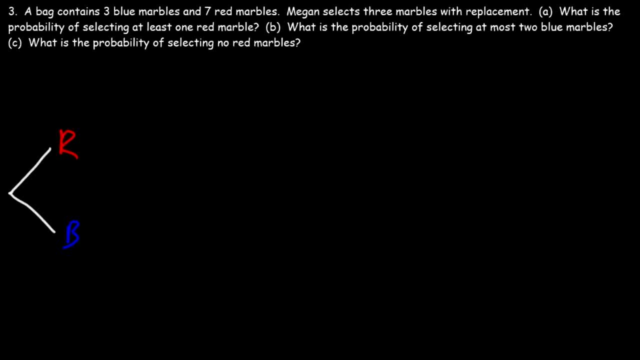 And on the second try, remember there's 3 selections. She's selecting 3 marbles, So on the second try, it can be red and blue again, And after selecting blue, it can also be red and blue again. Now there's a third try or a third selection. 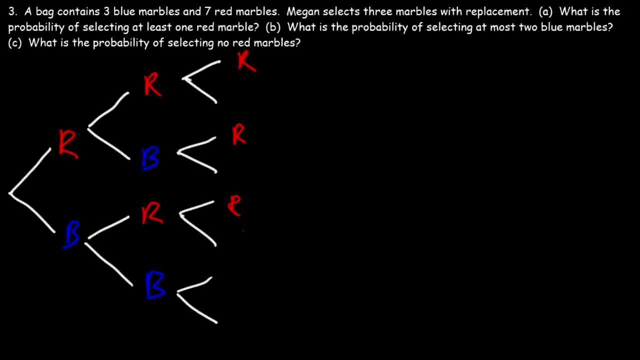 So it can be red or blue Or blue. So notice the possibilities. If we go in this direction, it can be R, R, R. Or if we travel in this direction, it can be R, R and then B. 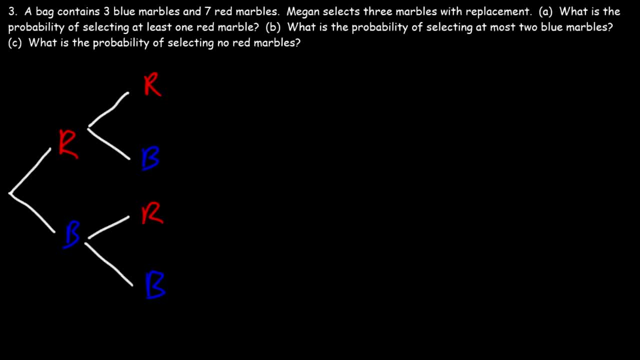 there's a third try or a third selection, so it can be red or blue. so notice the possibilities. if we go in this direction, it can be our, our, our, or if we travel in this direction, it can be our, our and then be. the next one is going to be our BR and then the. 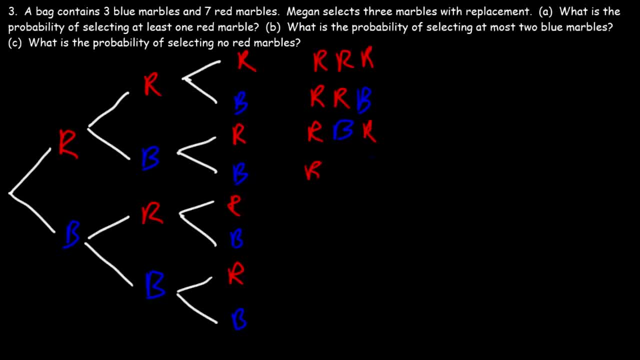 fourth option is our BB, and then the fifth option is: be our are, and then it's be be our, and then we have BB, are, and finally the last option, BBB. so we have eight different outcomes and the way you go about calculating that is that we have two choices- red or blue- and there's three selections, which is in three. 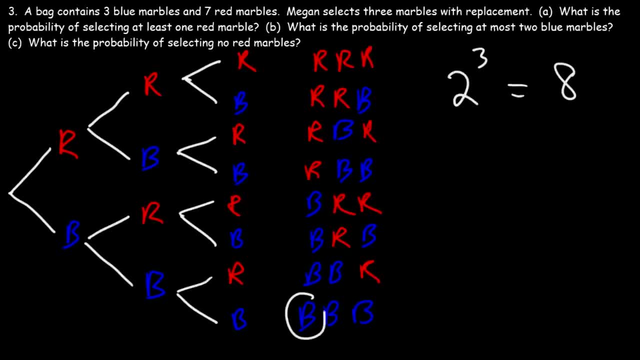 marbles. two to the third is eight. so in the selection we're choosing three marbles. two to the third is eight. so in the first selection is two options, red or blue, and the second selection two options, red or blue, so you multiply by two. and the third option. there's two options, red and blue. again two times two. 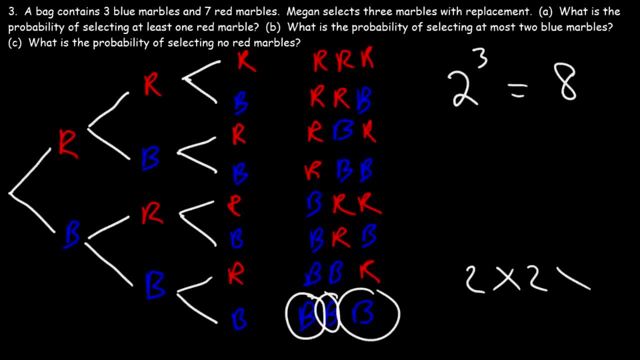 times two is eight, and so that's how we get a different outcomes. now let's answer. well, first we need to put down the probability values. so we have three blue marbles, seven red marbles. the probability of getting a red marble is seven over ten, and the probability of getting a blue marble is three over ten. 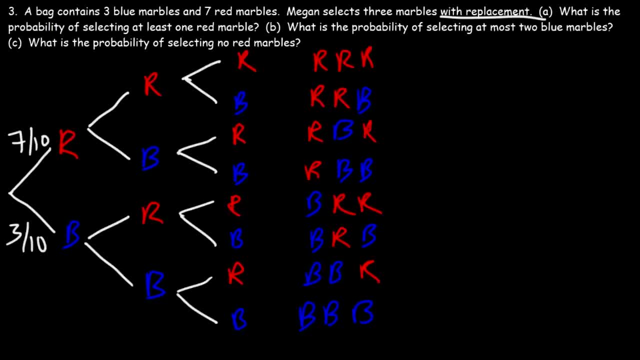 now, this is with replacement, which means that Megan is going to put the marble back in the back. so we're always going to have ten marbles, three blue marbles and seven red marbles. so every time she's selecting a red marble, the probability will be seven over ten. 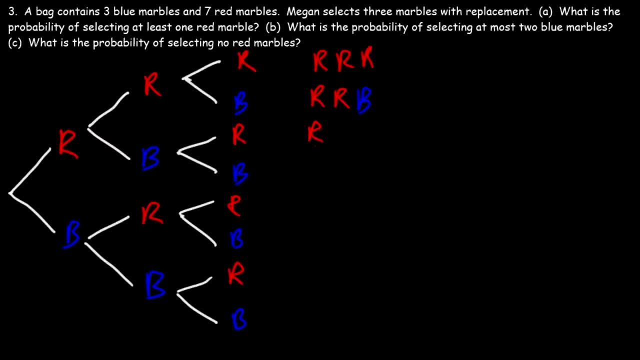 The next one is going to be R R, B R, And then the fourth option is R B B, And then the fifth option is B R R, And then it's B R B, And then we have B B R. 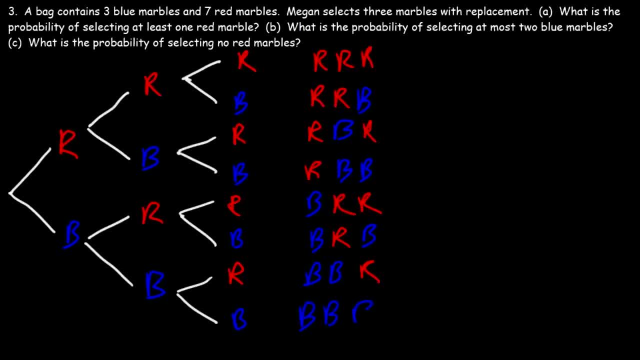 And then finally, the last option, B, B, B. So we have 8 different outcomes And the way you go about calculating that is that we have 2 choices- red or blue- And there's 3 selections. We're choosing 3 marbles. 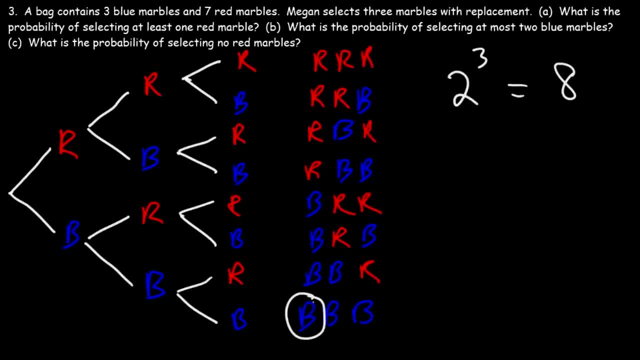 2 to the third is 8.. So in the first selection there's 2 options: red or blue. In the second selection 2 options, red or blue. So you multiply by 2.. In the third option there's 2 options. 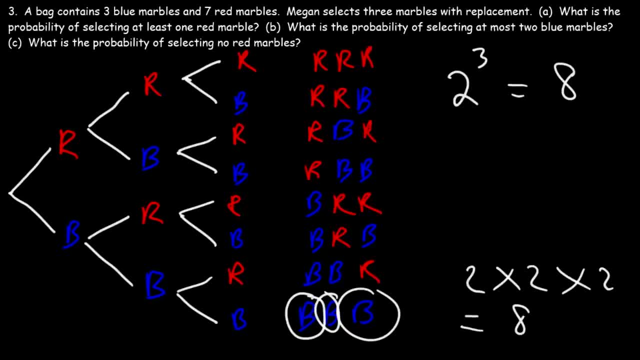 Red and blue again 2 times 2 times 2 is 8.. And so that's how we get 8 different outcomes. Now let's answer. Well, first we need to put down the probability values. So we have 3 blue marbles, 7 red marbles. 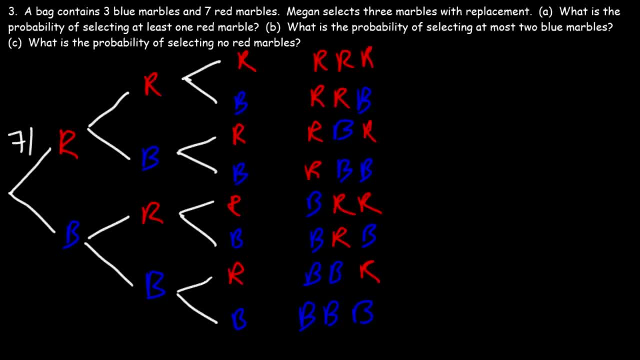 The probability of getting a red marble is 7 over 10.. And the probability of getting a blue marble is 3 over 10.. Now, this is with replacement, which means that Megan is going to put the marble back in the back. 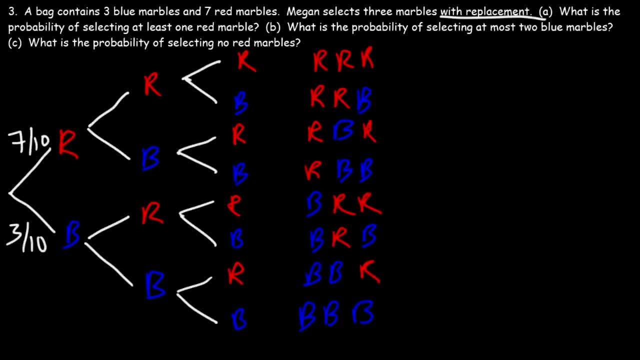 So we're always going to have 10 marbles: 3 blue marbles and 7 red marbles. So every time she's selecting a red marble, the probability will be 7 over 10.. And every time she selects a blue marble, the probability will be 7 over 10.. 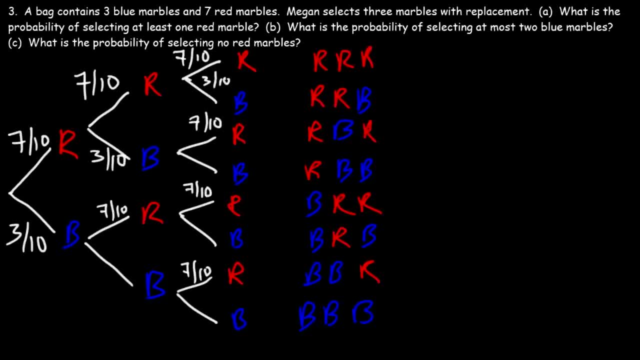 And every time she selects a blue marble, the probability will be 3 over 10.. So what is the probability of selecting at least 1 red marble? So let's identify all the outcomes that contain 1 red marble. So that would be these 7 outcomes. 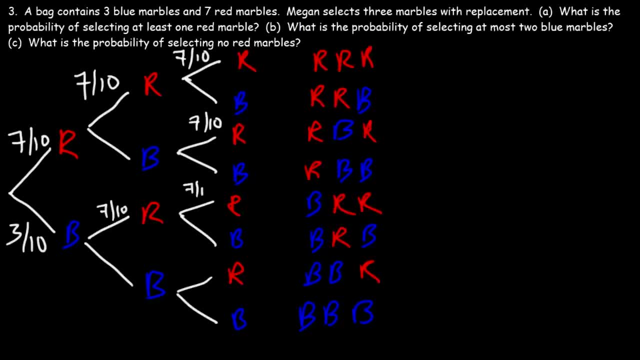 you, and every time she selects a blue marble, the probability will be three over ten. so what is the probability of selecting at least one red marble? so let's identify all the outcomes that contain one red marble. so that would be the seven, these seven outcomes. so now we can add up the probability of each of. 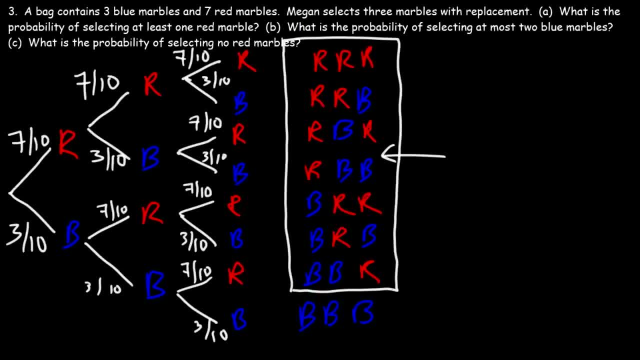 these seven events occurring. or we could say that the answer is equal to the probability. it's one minus the probability of this occurring you? so the probability of selecting at least one red marble is equal to the probability of not getting three blue marbles. so let's calculate the 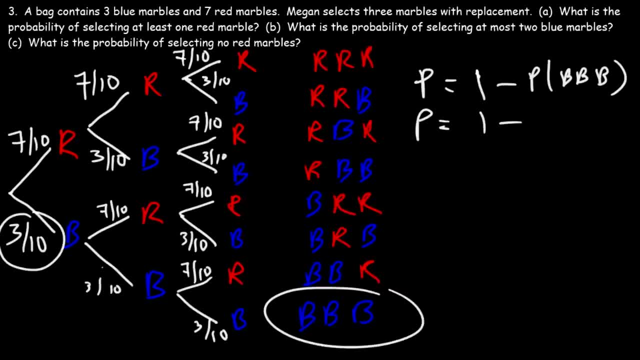 probability of getting three blue marbles. it's three over ten times two over ten times two over ten. so basically this is going to be three over ten, raised to the third power. three times three times three is twenty seven. ten times ten times ten times ten is a thousand and we need to get common denominators. 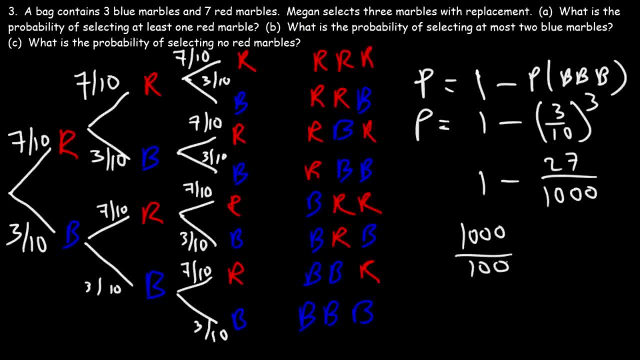 here one is the same as a thousand over a thousand. 1000 minus twenty seven is nine hundred and seventy three. so this is the answer as a decimal, its ninety seven point three percent. I mean as a percentage, as the decimals point nine seven three. so there's a ninety seven point three percent. 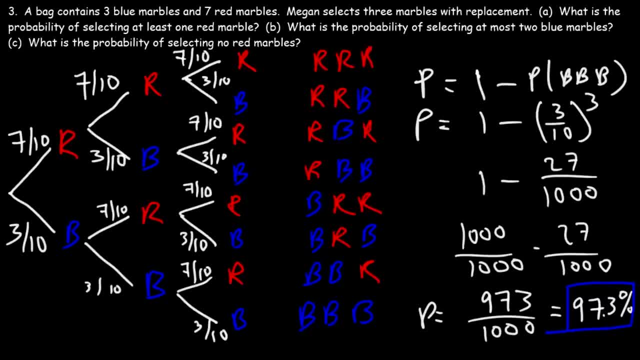 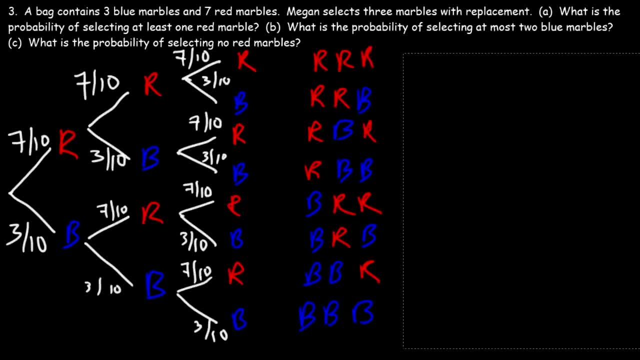 chance of selecting at least one red marble. now let's move on to Part B. what is the probability of selecting at most two blue marbles? so let's identify all of the outcomes with at most two blue marbles. so what does that mean? at most can we have three blue marbles? nope, the maximum is two blue marbles. so this: 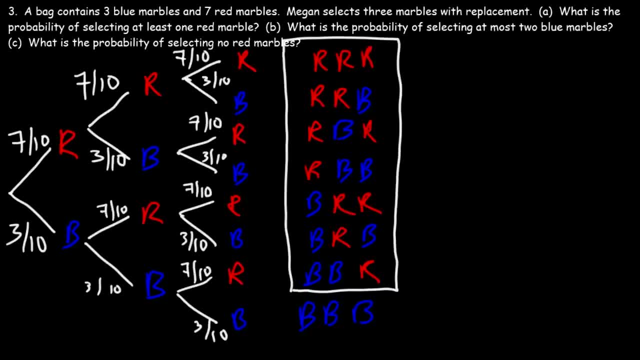 So now we can add up the probability of each of these 7 events occurring, Or we could say that the answer is equal to the probability. It's 1 minus the probability of this occurring. So the probability of selecting at least 1 red marble. 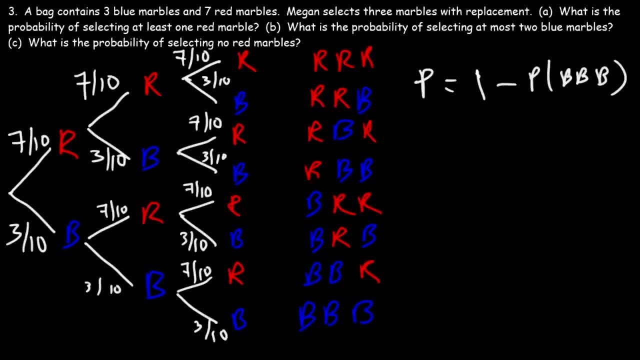 Selecting at least 1 red marble is equal to the probability of not getting 3 blue marbles. So let's calculate the probability of getting 3 blue marbles. It's 3 over 10 times 2 over 10 times 2 over 10.. 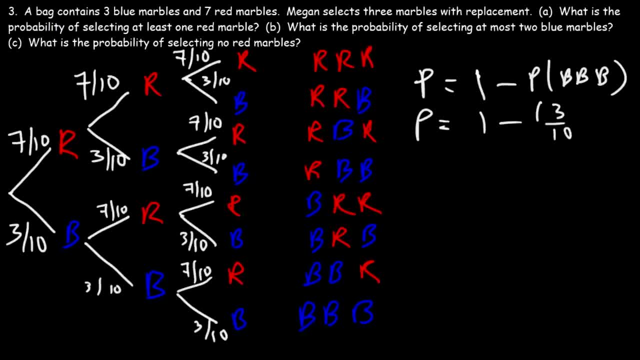 So basically this is going to be 3 over 10 raised to the third power. 3 times 3 times 3 is 27.. 10 times 10 times 10 is 1000.. And we need to get common denominators here. 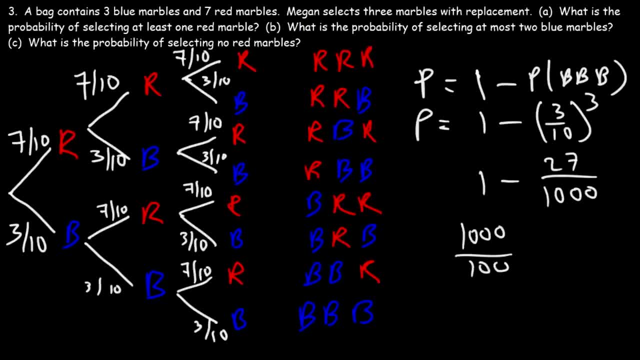 1 is the same as 1000 over 1000.. 1000 minus 27 is 973.. So this is the answer. As a decimal, it's 97.3%. I mean as a percentage. As a decimal, it's .973.. 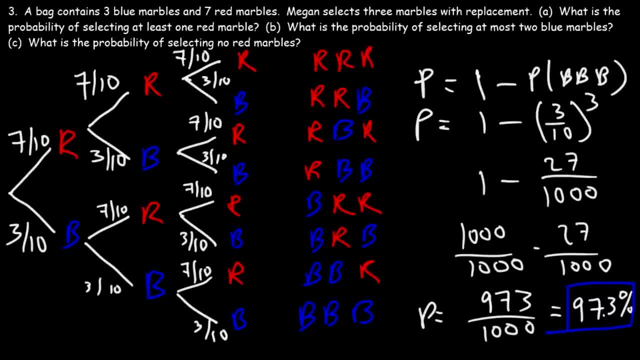 So there's a 97.3% chance of selecting at least 1 red marble. Now let's move on to Part B. What is the probability of selecting at most 2 blue marbles? So let's identify all of the outcomes with at most 2 blue marbles. 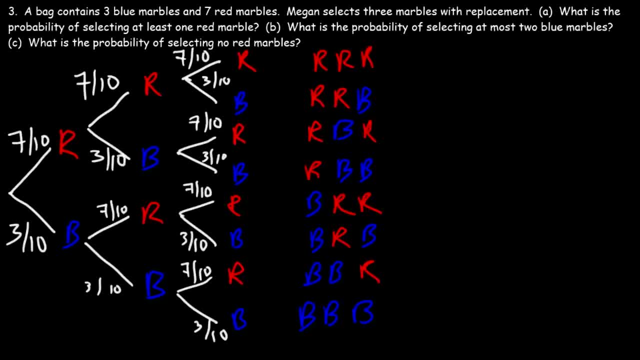 So what does that mean? at most Can we have 3 blue marbles? Nope, the maximum is 2 blue marbles. So this contains 2 blue marbles, This one too. This doesn't exceed 2 blue marbles. 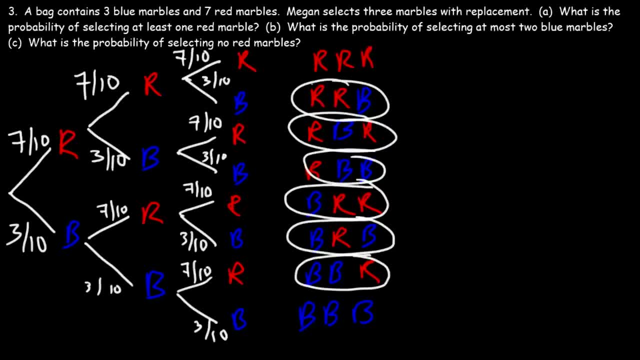 So that qualifies. What about the first option? Does that qualify? Well, let's think about it: At most 2 blue marbles. So that means that the maximum number of blue marbles is 2.. So we could have 2 blue marbles. 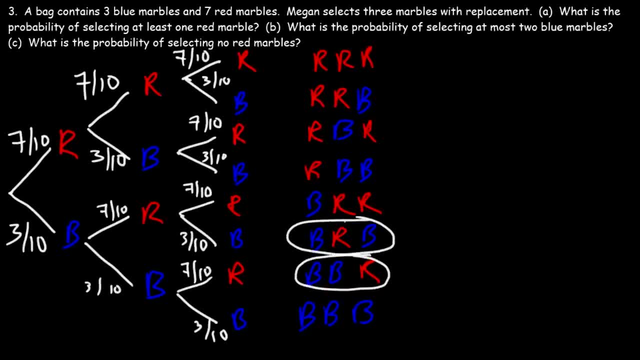 contains two blue marbles. this one too. this doesn't exceed two blue marbles, so that qualifies. what about the first option? does that qualify? well, let's think about it: at most two blue marbles. so that means that the maximum number of blue marbles is two, so we could have 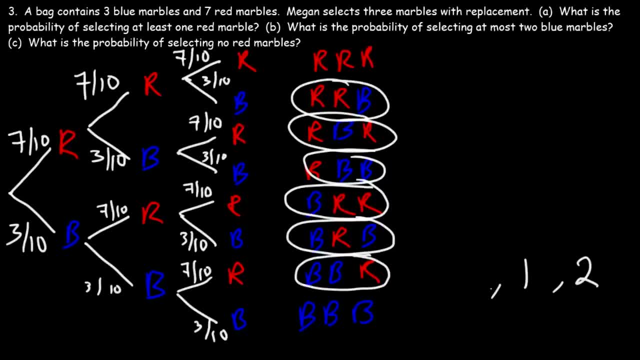 two blue marbles or anything less. we could have one blue marble or even zero blue marbles, because that's still less than two, so that option must be included. so once again, we're looking for the probability of getting these seven outcomes, which is equal to one minus the probability. 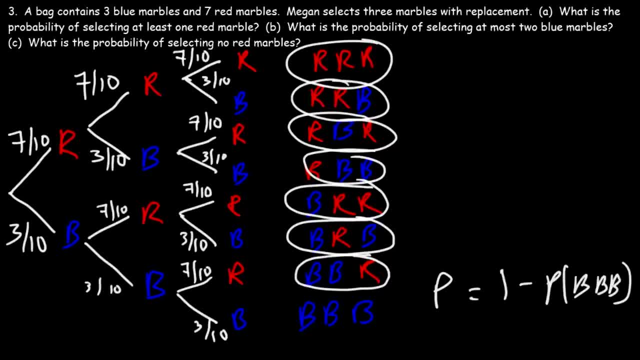 of getting three blues. so the answer for Part B is the same as that for Part A. it's going to be a ninety seven point three percent chance. the probability of selecting at least one red marble is the same as the probability of selecting at most two blue marbles. in both cases, this outcome is eliminated. now let's move on. 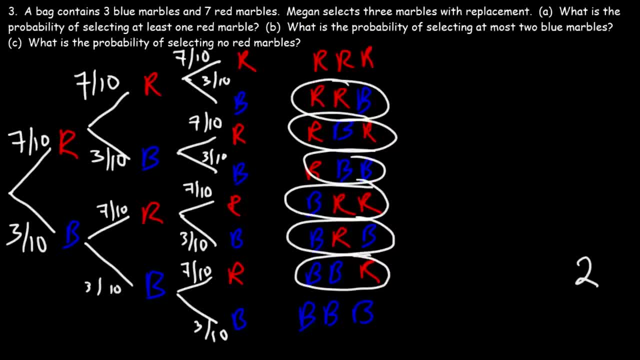 to Part C. what is the probability of selecting two no red marbles? this is the only option that has no red marbles, so we're just looking for the probability of getting all three blue marbles. so it's just going to be three out of ten, times itself three times, so that's 27 over 1,000. 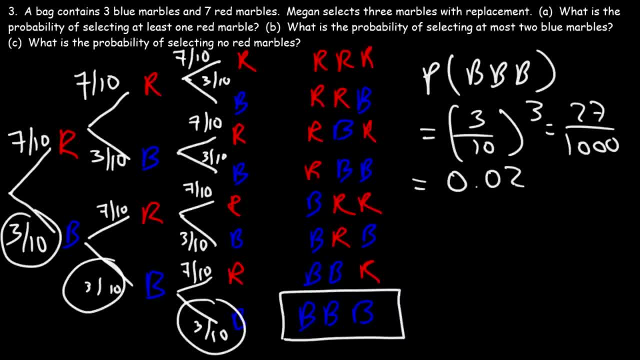 which, as a decimal, thats.027- and as a percentage, there's a 2.7% chance of this event occurring. Now I'm going to add a question to this: What is the probability of selecting two blue marbles? It has to be two. Go ahead and try that. That is exactly two blue. 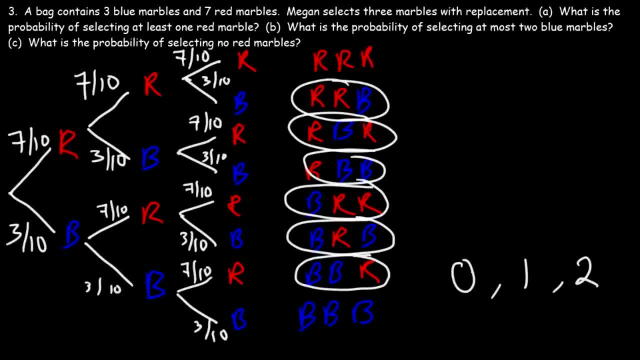 Or anything less. We could have 1 blue marble Or even 0 blue marbles, Because that's still less than 2.. So that option must be included. So once again, we're looking for the probability of getting these 7 outcomes. 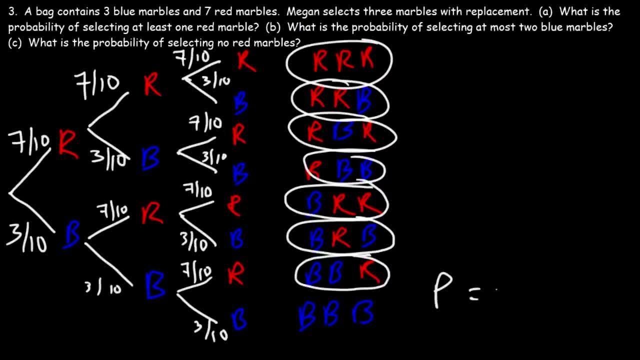 Which is equal to 1 minus the probability of getting 3 blues. So the answer for Part B is the same as that for Part A. It's going to be a 97.3% chance- The probability of selecting at least 1 red marble. 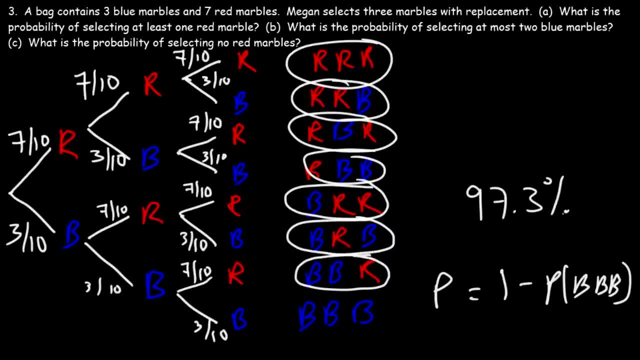 is the same as the probability of selecting at most 2 blue marbles. In both cases, this outcome is eliminated. Now let's move on to Part C. What is the probability of selecting no red marbles? This is the only option that has no red marbles. 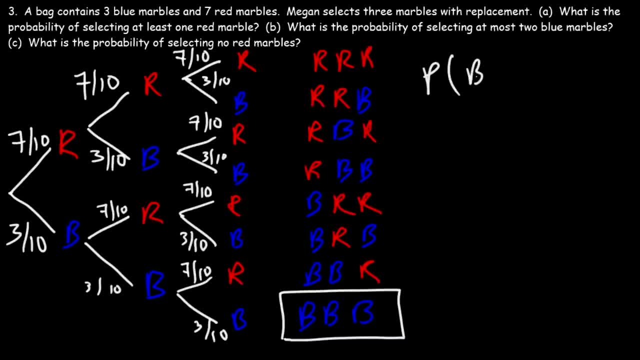 So we're just looking for the probability of getting all 3 blue marbles. So it's just going to be 3 out of 10, times itself 3 times. So that's 27 over 1000.. Which, as a decimal, that's .027.. 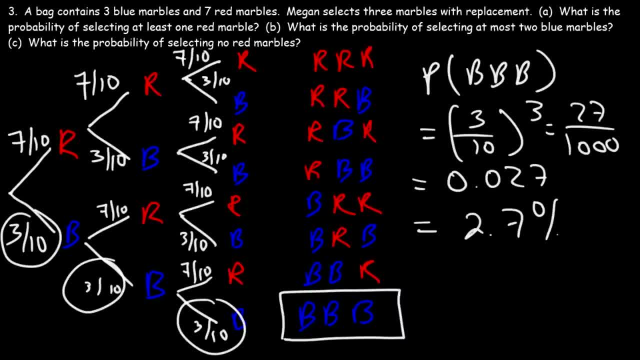 And as a percentage, there's a 2.7% chance of this event occurring. Now I'm going to add a question to this: What is the probability of selecting 2 blue marbles? It has to be 2.. 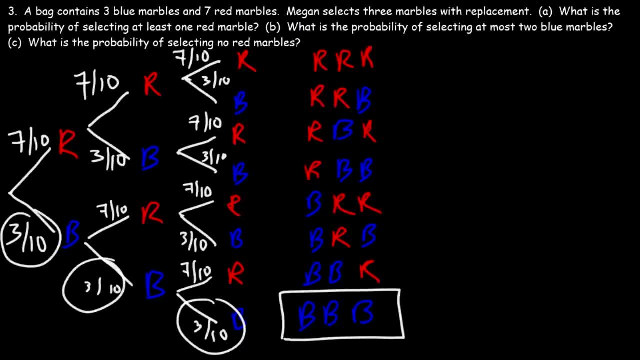 Go ahead and try that. That is exactly 2 blue marbles. So we need to highlight all the options with 2 blue marbles. So that's this one, That's one, Here's another one And here is the second one. 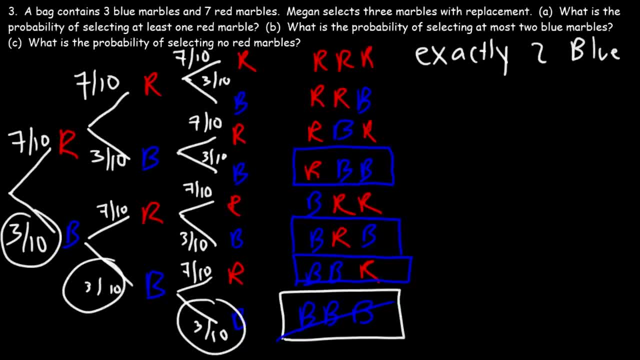 But not this one. So we need to find the probability of getting these 3 events and then we're going to add them. So the probability of getting a red and then a blue and then a blue is going to be 7 over 10.. 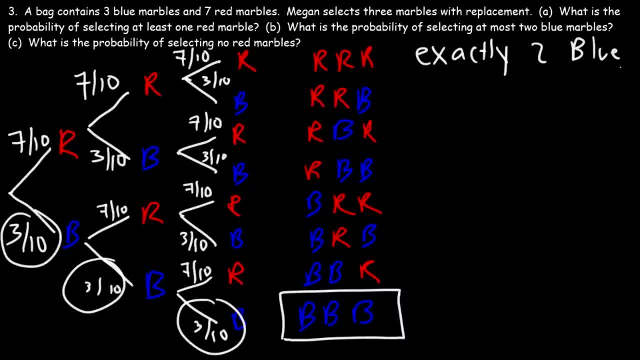 marbles. So we need to highlight all the options with two blue marbles. So that's this one, That's one, Here's another one, And here is the second one, but not this one. So we need to find the probability. 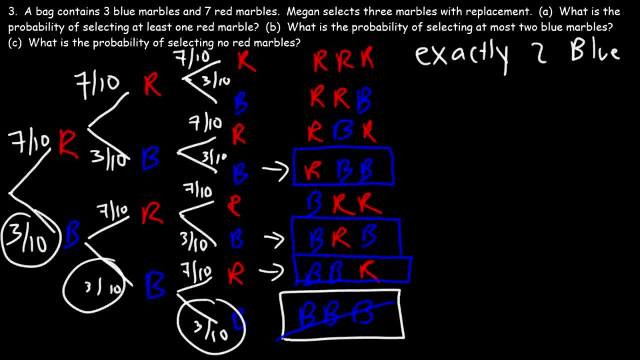 of getting these three events and then we're going to add them. So the probability of getting a red and then a blue and then a blue, It's going to be 7 over 10 times 3 over 10 times 3 over 10.. So 3 times 3 is 9,. 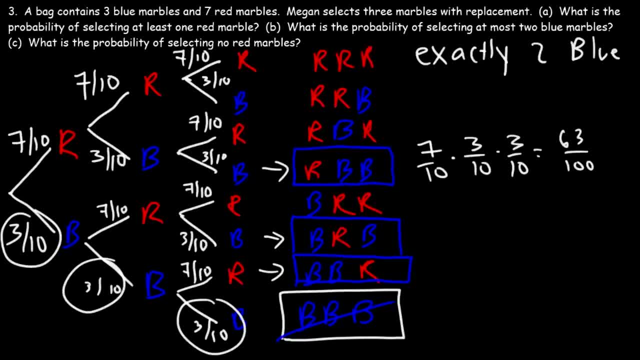 is 63.. So that's 63 over 1,000.. Now, for this one it's going to be the same, Because the probability of getting a blue is 3 over 10, for a red is 7 over 10,. 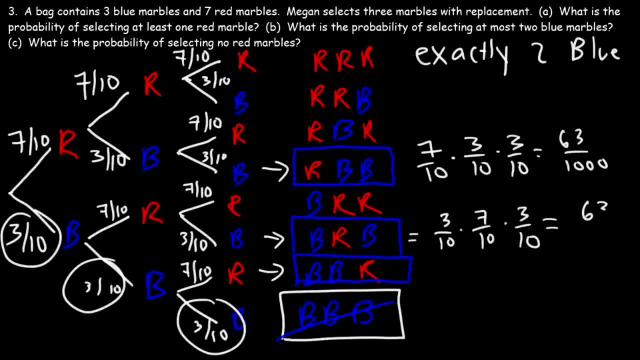 and then 3 over 10 for another blue, So that's still going to be 63 over 1,000. And the same is true for this one too. To get the first blue is 3 out of 10, the second blue is. 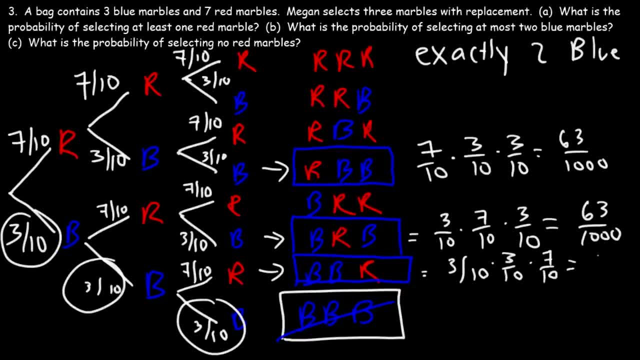 3 out of 10, and the red is 7 out of 10.. So we're going to add up 63 three times, or 63 times 3,, that's 189.. So it's 189 over 1,000, which is 0.189.. 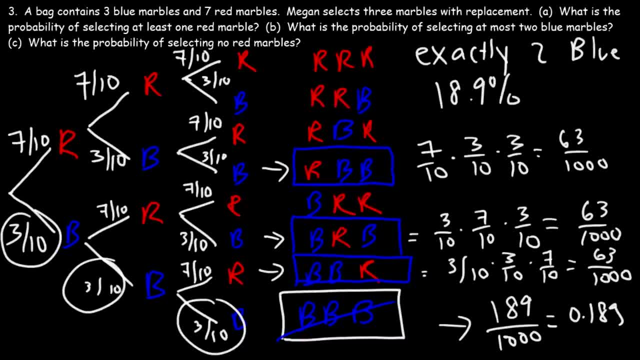 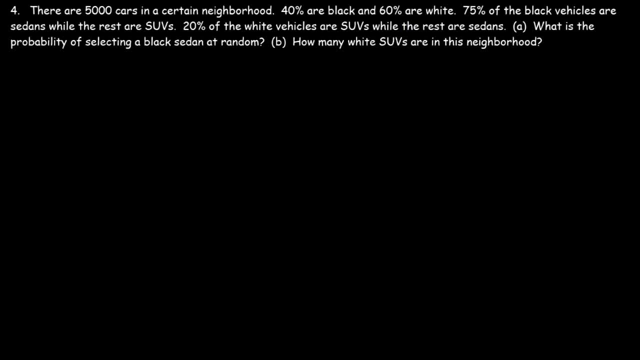 So there is an 18.9% chance of getting exactly two blue marbles. Now let's work on this problem. There are 5,000 cars in a certain neighborhood. 40% are black And 60% are white. 75% of the black. 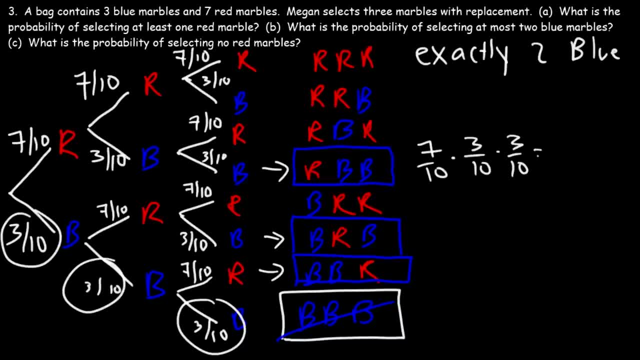 times 3 over 10.. times 3 over 10.. So 3 times 3 is 9.. 9 times 7 is 63. So that's 63 over 1000.. Now for this one. it's going to be the same. 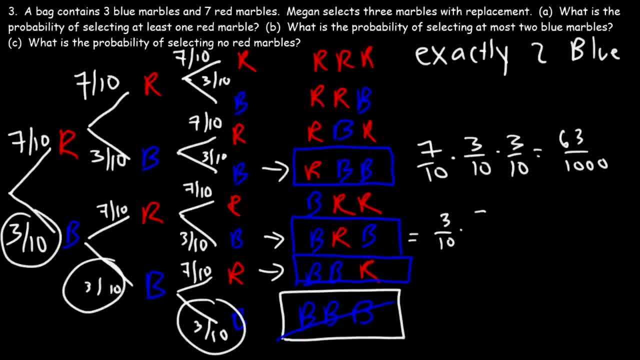 Because the probability of getting a blue is 3 over 10.. For a red is 7 over 10. And then 3 over 10. for another blue. So that's still going to be 63 over 1000.. 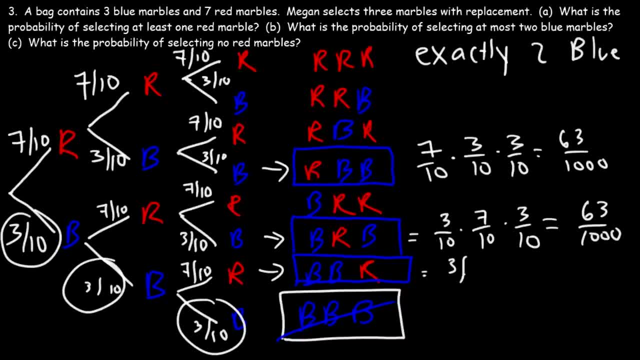 And the same is true for this one too, To get. the first blue is 3 out of 10.. The second blue is 3 out of 10. And the red is 7 out of 10.. So we're going to add up 63.. 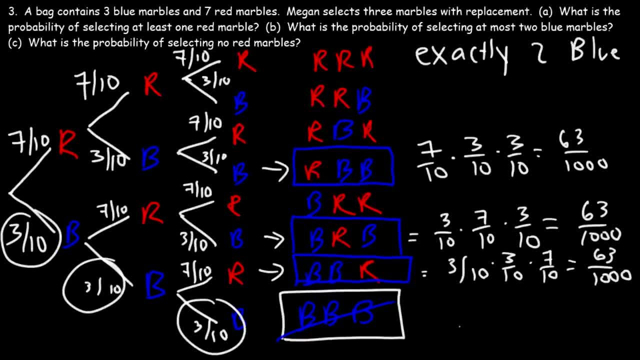 3 times or 63 times 3. That's 189.. So it's 189 over 1000.. which is .189.. So there is an 18.9% chance of getting exactly 2 blue marbles. 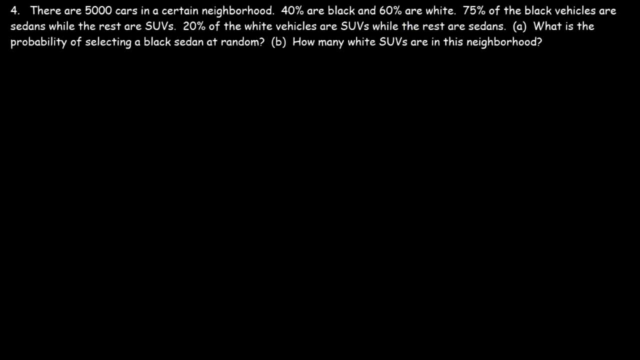 Now let's work on this problem. There are 5000 cars in a certain neighborhood. 40% are black and 60% are white. 75% of the black vehicles are sedans, While the rest are SUVs. 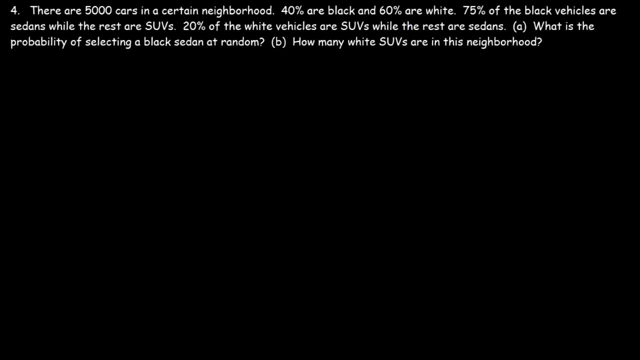 20% of the white vehicles are SUVs, While the rest are sedans. What is the probability of selecting a black sedan at random? So let's begin. There's 5000 cars in this neighborhood, So out of that. 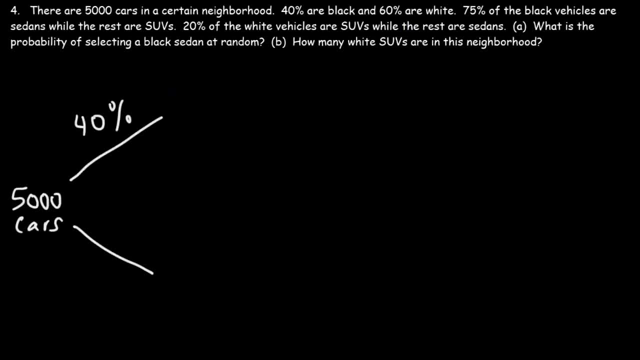 40% of those cars are black And the other 60% is going to be white. So what is 40% of 5000?? 40% of 5000. is basically .40. times 5000.. 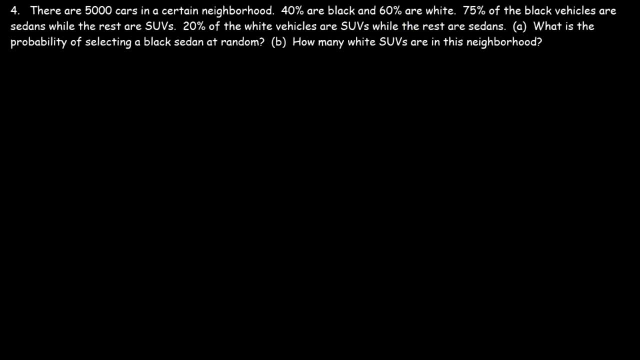 vehicles are sedans, while the rest are SUVs. 20% of the white vehicles are SUVs, while the rest are sedans. What is the probability of selecting a black sedan at random? So let's begin. There's 5,000 cars in this neighborhood. 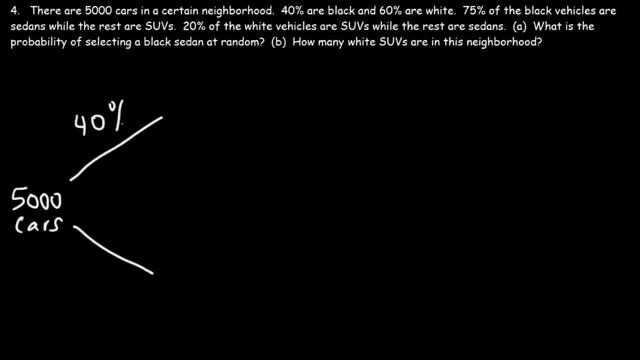 So out of that, 40% of those cars are black and the other 60% is going to be white. So what is 40% of 5,000?? 40% of 5,000 is basically 0.40 times 5,000. And so that's going to be 2,000.. 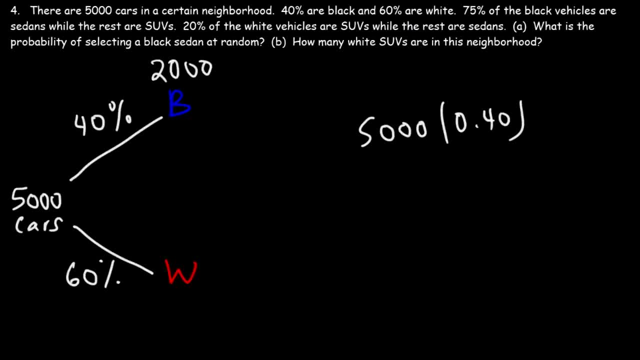 So that's going to be 2,000.. So that's going to be 2,000.. So there's 2,000 black cars. 60% of 5,000 is 3,000.. So we have 3,000 white cars. 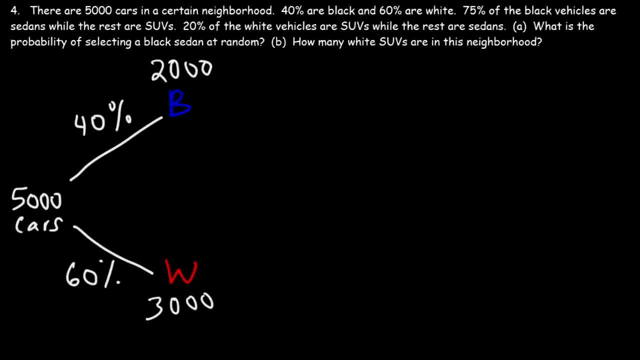 in the neighborhood Now, 75% of the black vehicles are sedans, So let me create another tree diagram. So this will be 75%, which means this part has to be 25% because it has to add up to 100.. 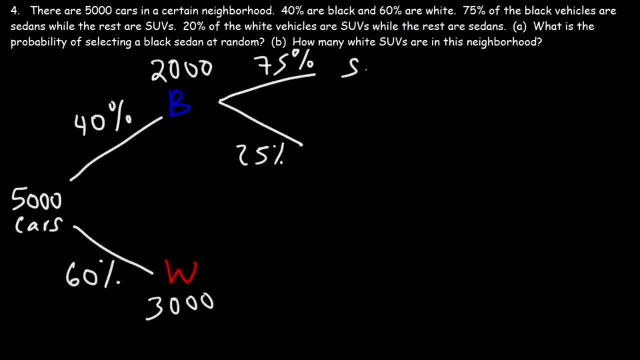 So this is for the sedans and the other 25% has to be SUVs. So 25% of 2,000 is 500, and 75% of 2,000 has to be 1,500, because these two numbers 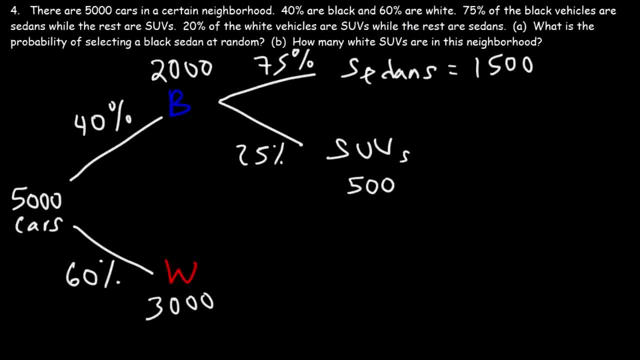 have to add up to 2,000.. So this is for the sedans. transformation, which means the number of spaces and the number of all the different buildings you're seeing, and except for the seats, there are 72.. Now for the white vehicles: 20% are SUVs. 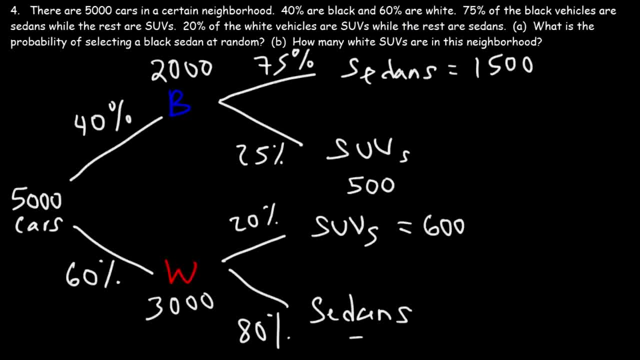 which means the other 80% has to be sedans. Now, 20% of 3,000.. That's 3,000 times 0.20.. 3,000 times 0.8, that's going to give us 2,400 white sedans. 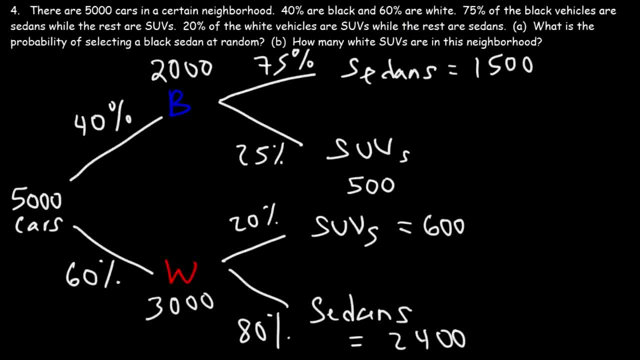 So now we can answer the questions. What is the probability of selecting a black sedan at random? So how many black sedans do we have? So this is where the black sedans are. There's 1,500 black sedans in the neighborhood, out of 5,000 cars. 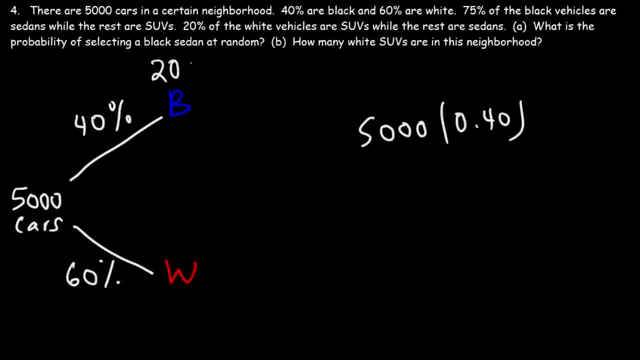 And so that's going to be 2000.. So there's 2000 black cars, 60% of 5000. is 3000. So we have 3000 white cars in the neighborhood Now, 75% of the black vehicles. 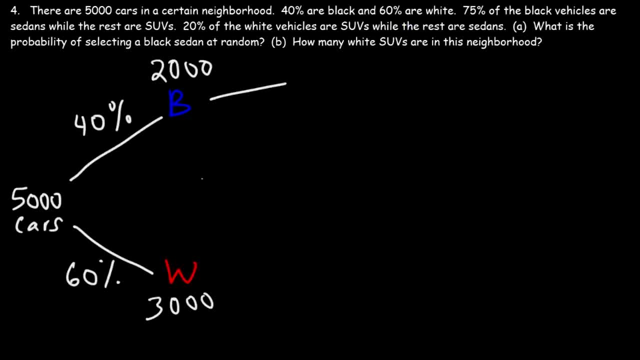 are sedans, So let me create another tree diagram. So this will be 75%, Which means this part has to be 25% Because it has to add up to 100.. So let's. So. this is for the sedans. 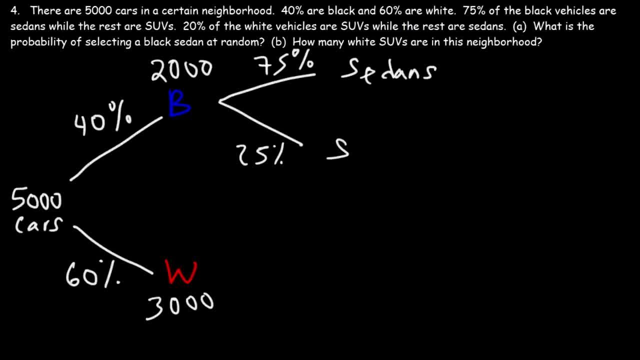 And the other 25% has to be SUVs. So 25% of 2000. is 500. And 75% of 2000. has to be 1500. Because these two numbers 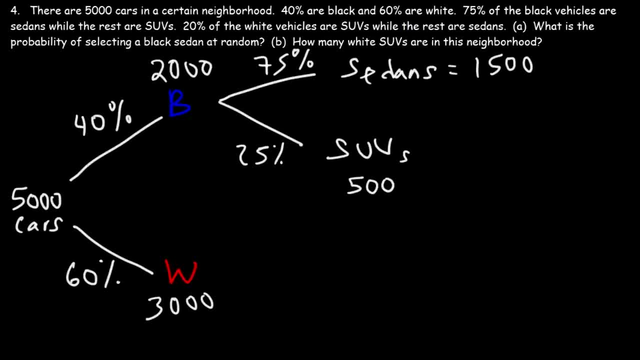 have to add up to 2000.. Now for the white vehicles. 20% has to be our SUVs, Which means the other 80% has to be sedans. Now, 20% of 3000.. That's 3000.. 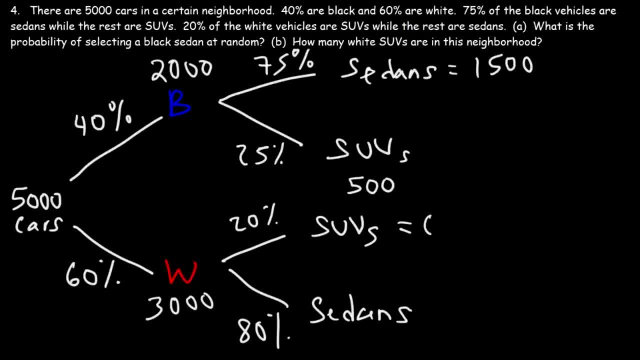 times .20.. That's going to give us 600 SUVs And 80% of 3000.. or 3000 times .8.. That's going to give us 2400 white sedans. So now we can answer the questions. 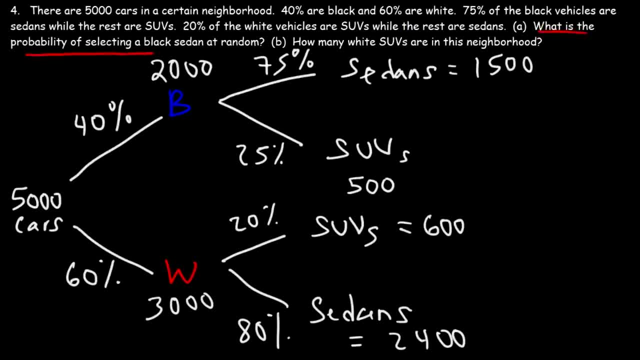 What is the probability of selecting a black sedan at random? So how many black sedans do we have? So this is where the black sedans are. There's 1500 black sedans in the neighborhood out of 5000 cars. 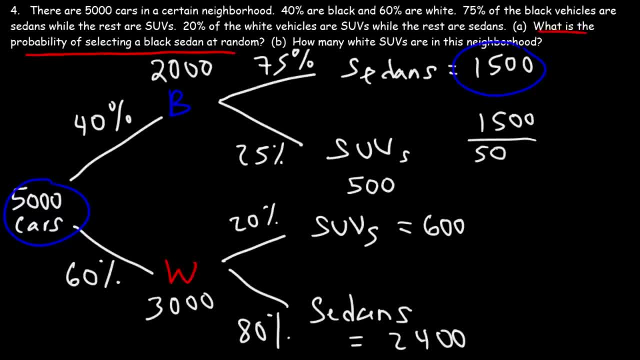 So it's going to be 1500.. divided by 5000.. And so, as a decimal, that's .3. Which is 30%. So there's a 30% chance of selecting a black sedan at random. 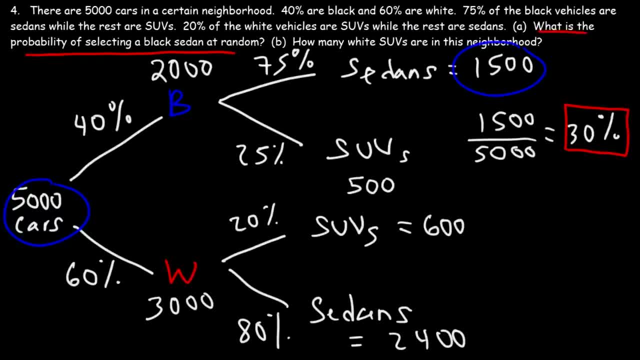 Now there's another way in which you can get that same answer, And it's by multiplying these two percentages. So if you multiply .4.. by .75.. it will give you .3. Which is equal to 30%. If you multiply .3 by 100..